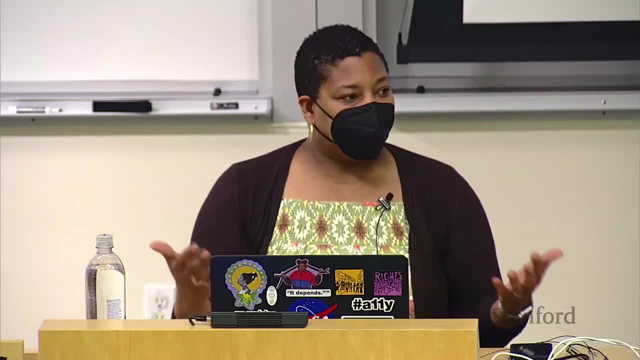 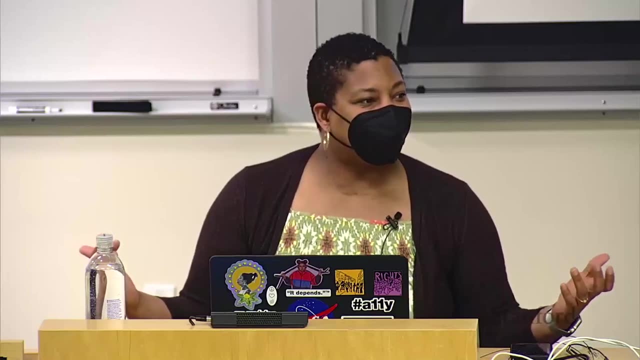 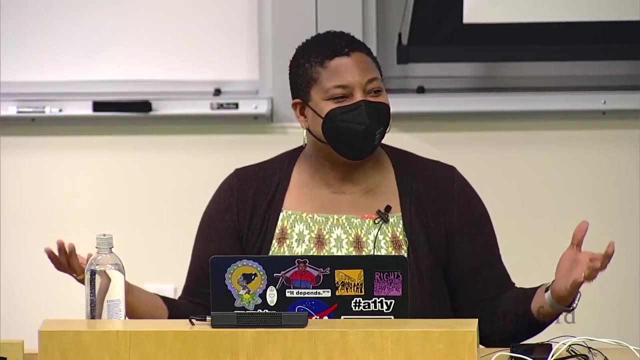 and Gus is blind. And when I mentioned to Gus you know what Pokemon was and I was describing it for those who don't know. does anybody in here want to describe it? Because I always like to ask who? who are my Pokemon Go players? Come on, No one wants to describe it. 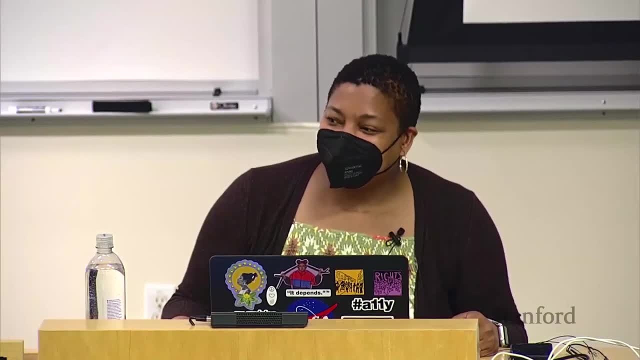 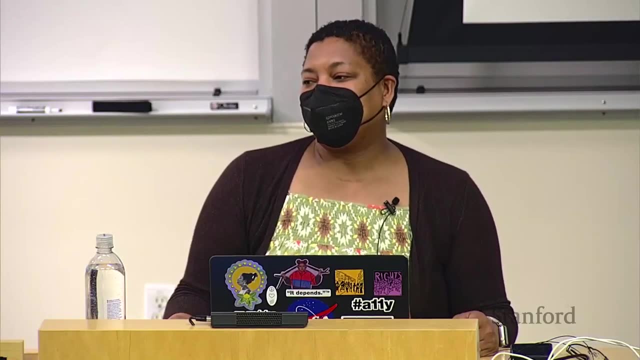 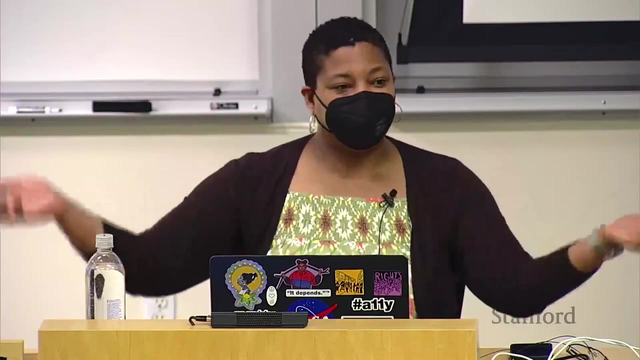 Yeah, it's a game that, that is, that has like the real-life map on the app and you're supposed to like walk around to different locations in real life to catch things. Yeah, so it has a real-life map. It's using augmented reality, right, And you use it to you catch things, right, And so I was describing to. 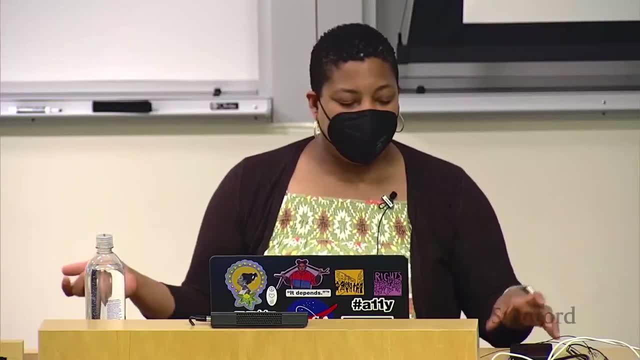 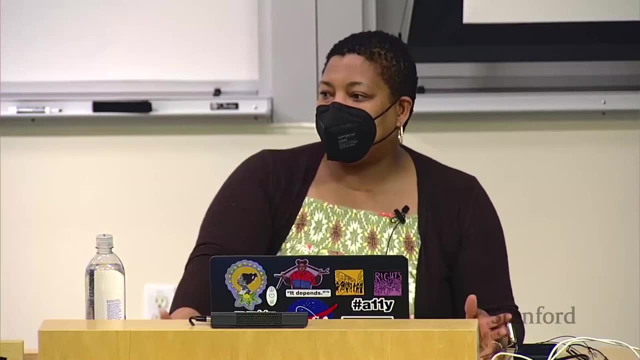 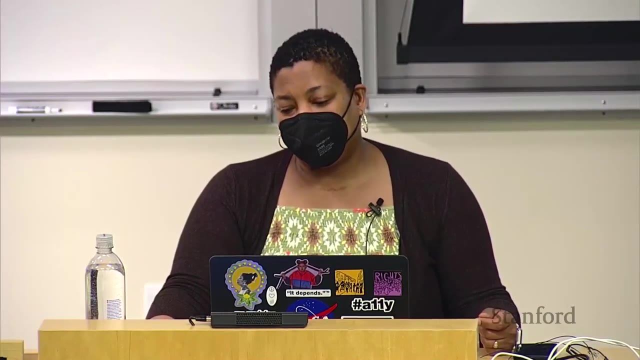 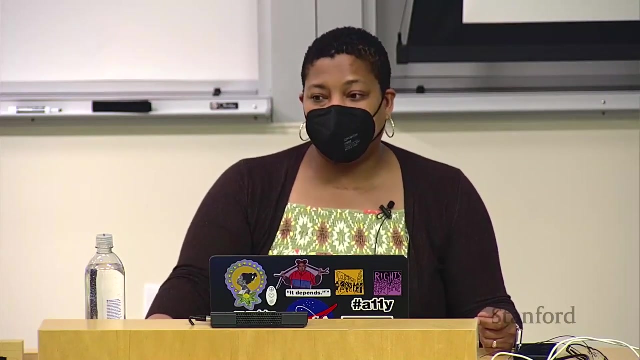 Gus the game and how, how you play. and he said I wish I could play. And I thought: why can't he play? Because he's blind. he can't That. that made no sense to me, And so one of the things that I decided to do this was right before I was going to teach a summer class. I said I'm going to have my students work on a project to create a concept for an augmented reality experience for someone who is blind. 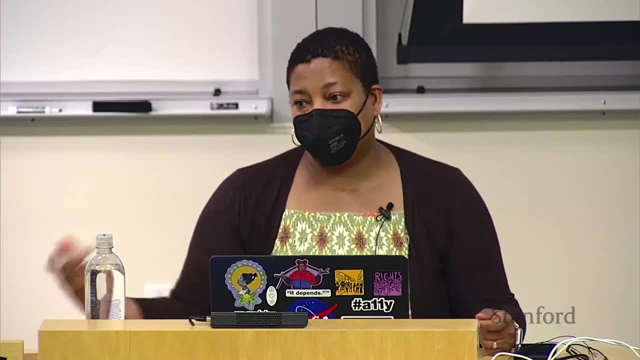 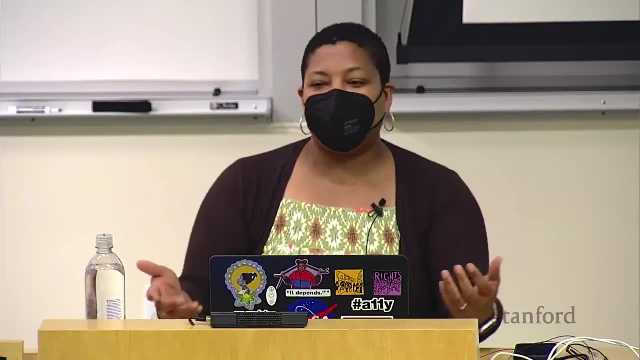 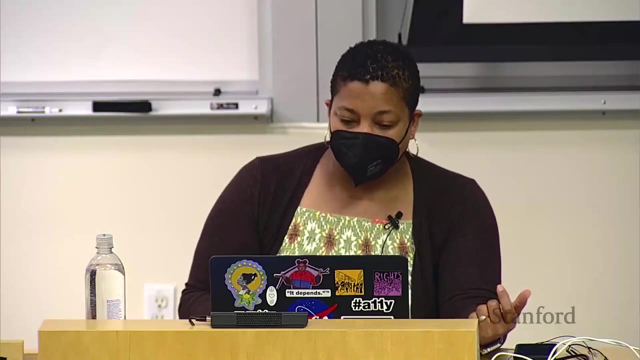 And so my students worked with Gus and they also got to work with people in the blind community and they came up with several different concepts. So this is my story of telling you how I got interested in accessibility and inclusion in the space of XR. 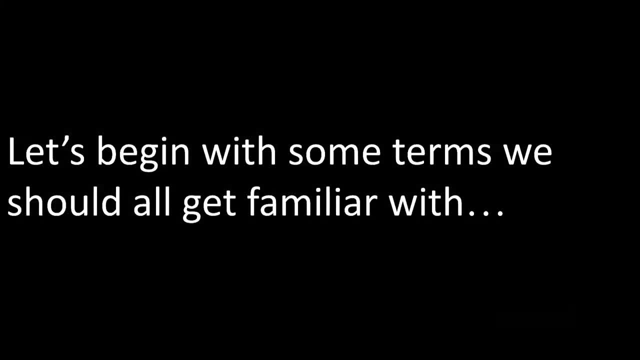 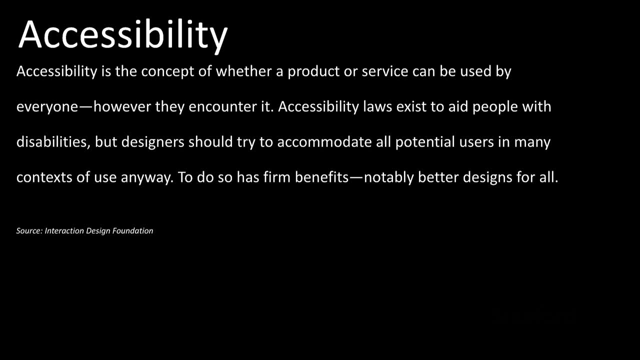 So I want to first start with some terms we should all get familiar with. The first one is accessibility. Some of you may know what accessibility is, some of you may not. Accessibility is concept of whether a product or service can be used by everyone, however they. 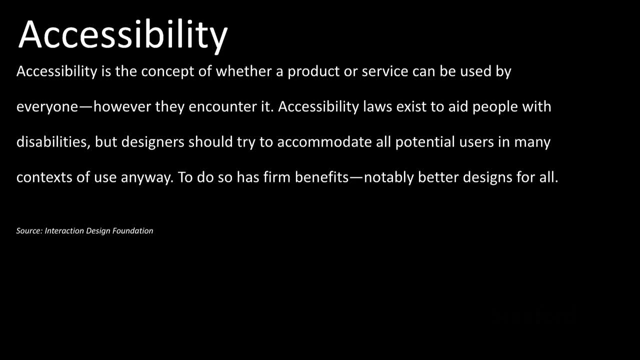 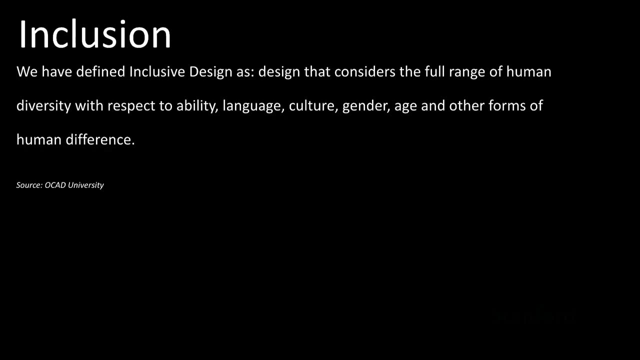 encounter it. accessibility laws exist to aid people with disabilities, but designers should try to accommodate all potential users in many contexts of use anyway. to do this has firm benefits, notably better designs for all. next is inclusion. now you'll hear me say this description, but really don't leave. 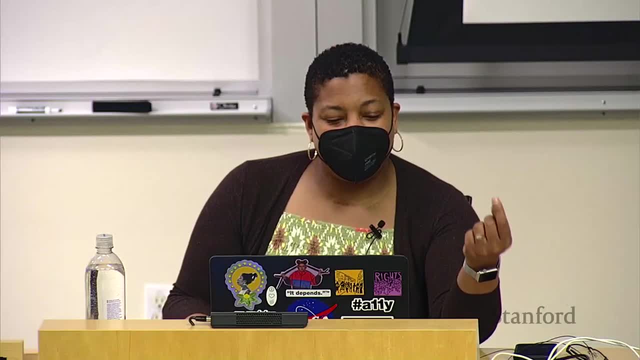 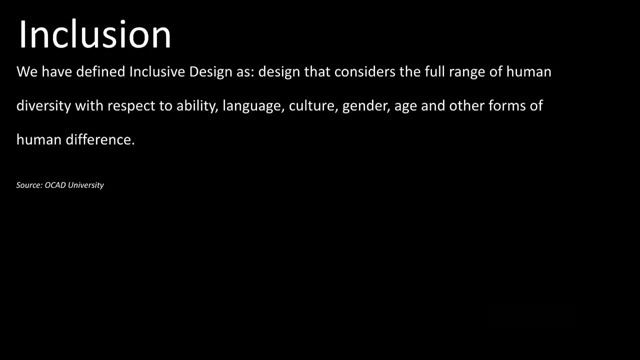 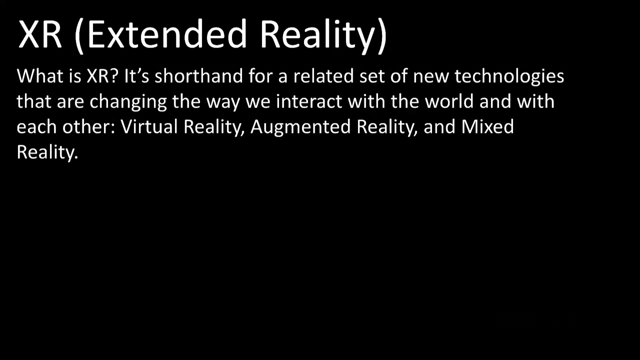 people out, I don't know how else to say it- we have defined- this is from OCAD University- we have defined inclusion design as design that considers the full range of human diversity with respect to ability, language, culture, gender, age and other forms of human difference, and XR. so XR is stands for extended reality. it's 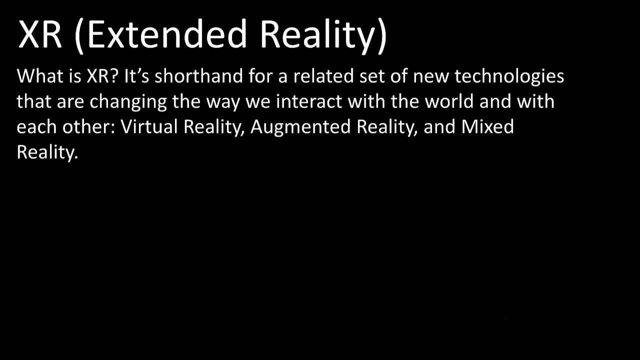 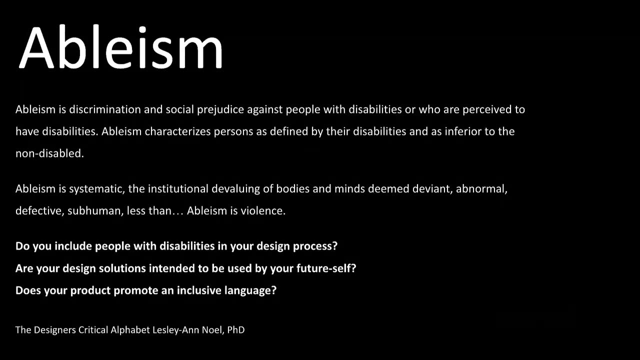 shorthand for a related statement. so this is a set of technologies that are changing the way we interact with the world and with each other. so this is virtual reality, augmented reality and mixed reality. next is ableism. this is a very important term for folks to know and understand because it is at the root of so many things that are broken. 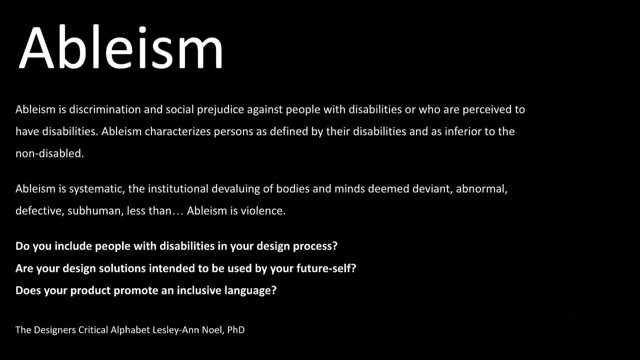 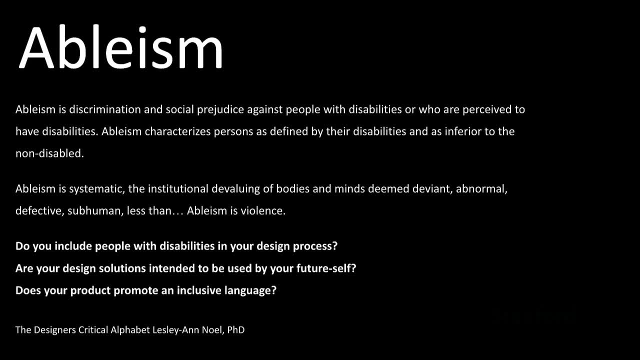 the institutional devaluing of bodies and minds deemed deviant, abnormal, defective, subhuman. less than ableism is violence. so questions to ask as you're working on things are: do you include people with disabilities in your design process? are your design solutions intended to be used by your future self? does your 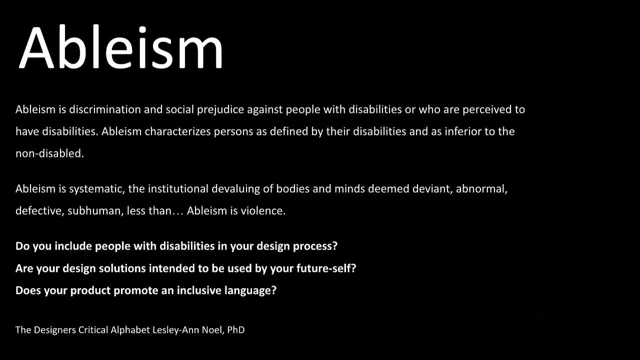 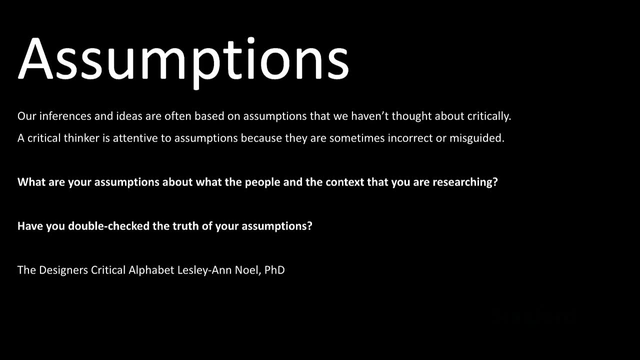 product. promote an inclusive language. next is assumptions. we all have them, right. there are inferences, and ideas are often based on assumptions that we haven't thought about critically. a critical thinker is attentive to assumptions because they are sometimes incorrect or misguided. so questions to ask yourself are: what are your assumptions about the people and 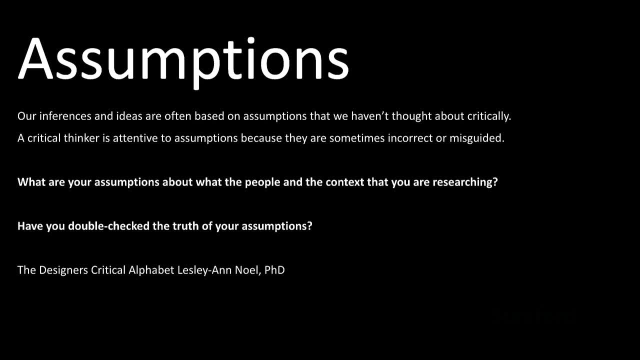 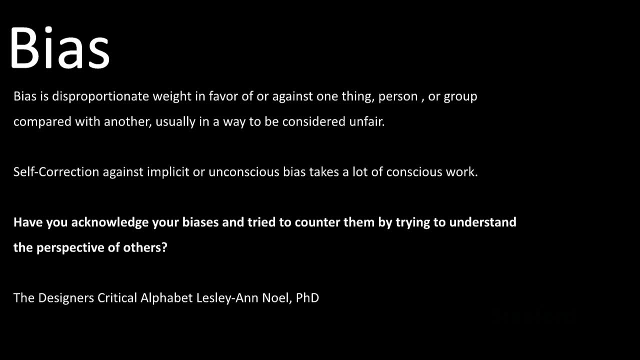 context that you are researching. have you double checked the truth of your assumptions? next is bias. bias is disproportionate weight in favor of or against one thing, person or group compared with another, usually in a way to be considered unfair. self-correction against implicit or unconscious bias takes a lot of conscious. 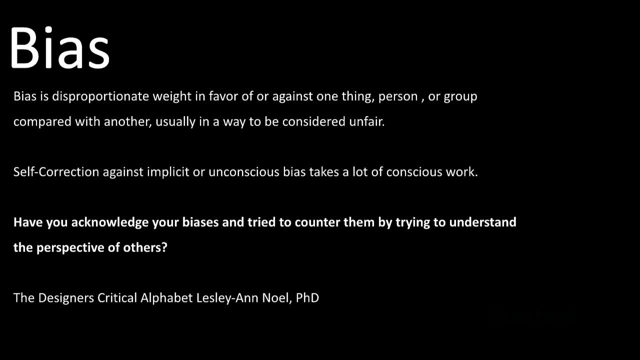 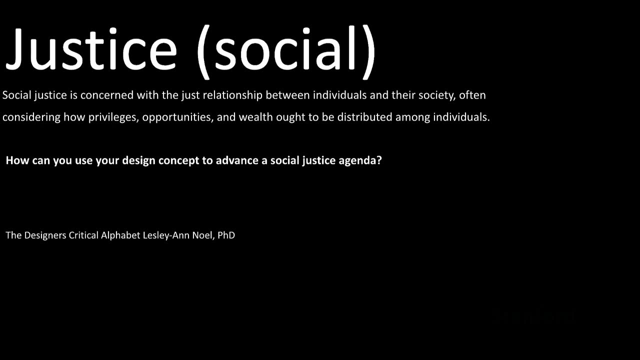 work. so question is: have you acknowledged your biases and try to counter them by trying to understand the perspective of others? next is justice, social justice. so social justice is concerned with the just relationship between individuals in their society. often people who are not aware of the social justice system consider how privilege is opportunities and wealth ought to be. 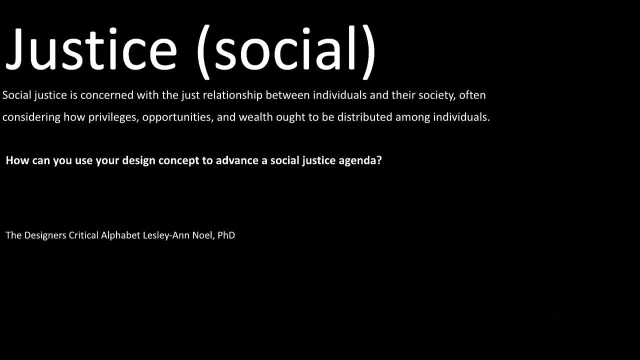 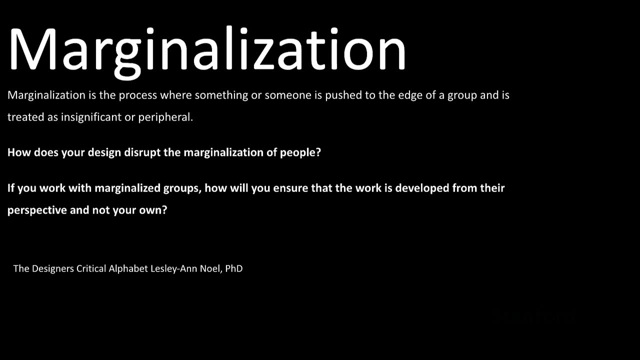 distributed among individuals. question to ask is: how can you use your design concept to advance a social justice agenda: marginalization? so marginalization is a process where something or someone is pushed to the edge of a group and is treated as insignificant or peripheral. so questions to ask are: how does your 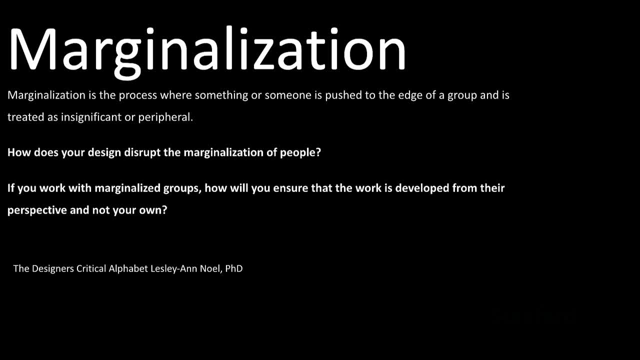 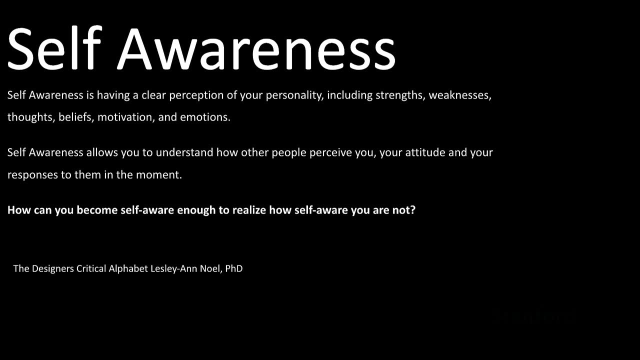 design disrupt the marginalization of people. If you work with marginalized groups, how will you ensure that the work is developed from their perspective and not your own Self-awareness? I cannot stress this enough for designers. I encourage it to my students so much to know yourself. It is so. 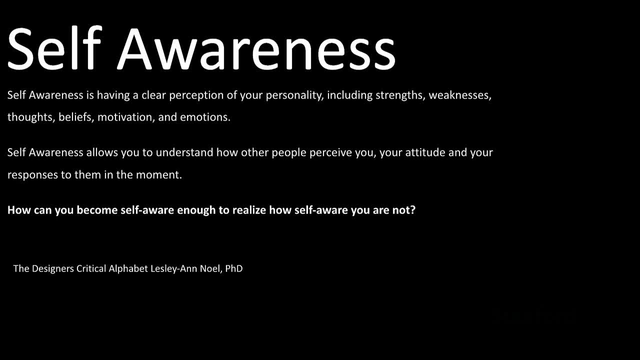 important Self-awareness is having a clear perception of your personality, including strengths, weaknesses, thoughts, beliefs, motivations and emotions. Self-awareness allows you to understand how other people perceive you, your attitude and your responses to them in the moment. Question to ask is: how can you become self-aware enough to realize how self-aware 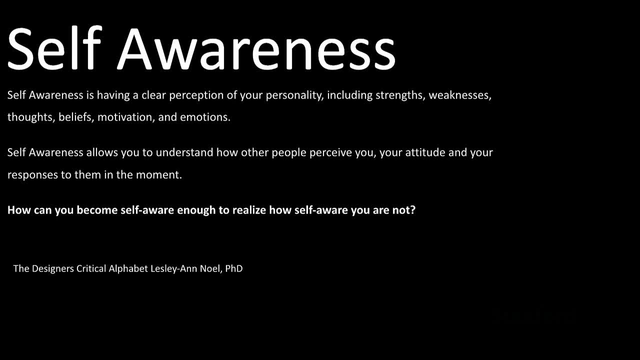 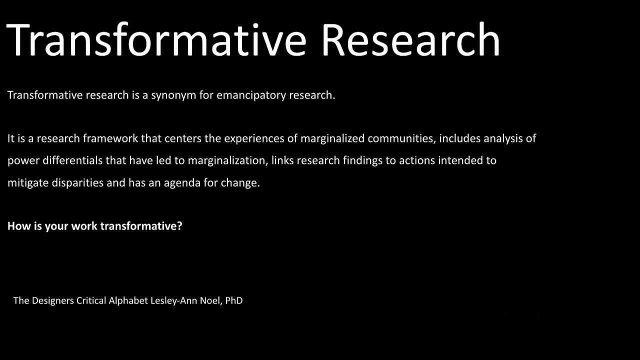 you are not Transformative research. Transformative research is a synonym for emancipatory research. It is a research framework that centers the experiences of marginalized communities, including analysis of power differentials that have led to marginalization, links research findings to actions intended to 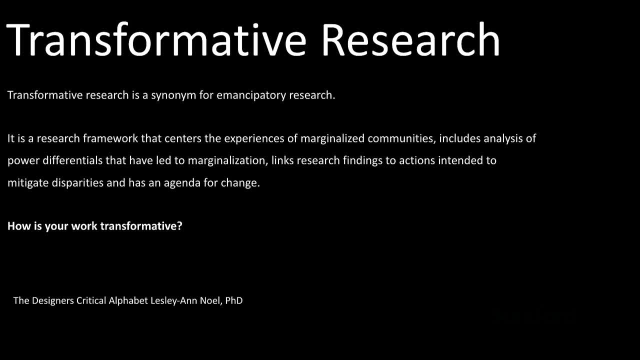 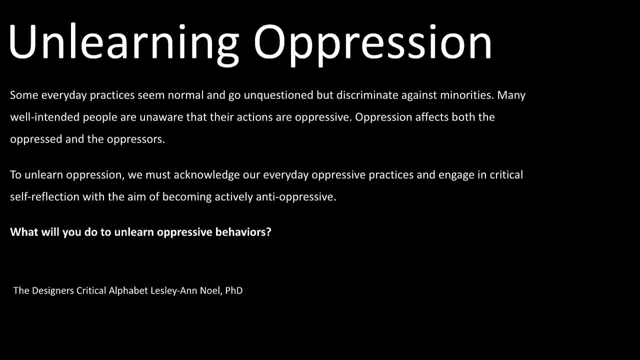 mitigate disparities and has an agenda for change. Question to ask is: how is your work transformative? Unlearning oppression? Some everyday practices seem normal and go unquestioned, but discriminate against minorities. Many well-intended people are unaware that their actions are oppressive. 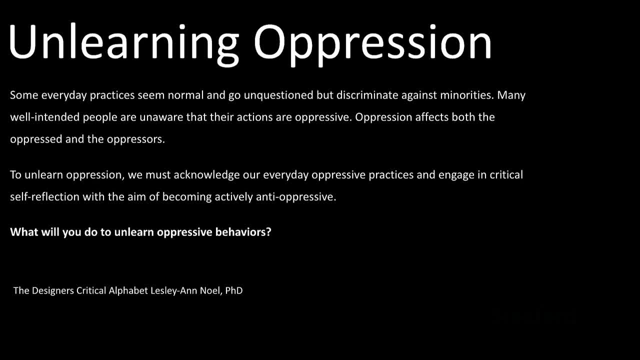 Oppression affects both the oppressed and the oppressor. To unlearn oppression, we must acknowledge our everyday oppressive practices and engage in critical self-reflection with the aim of becoming self-aware. Unlearning oppression is a synonym for emancipatory research. It is also a way of being actively anti-oppressive. 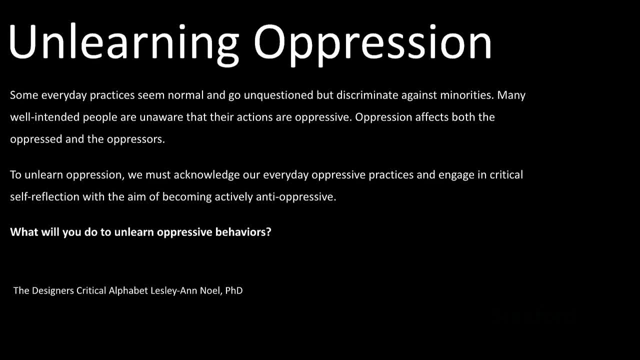 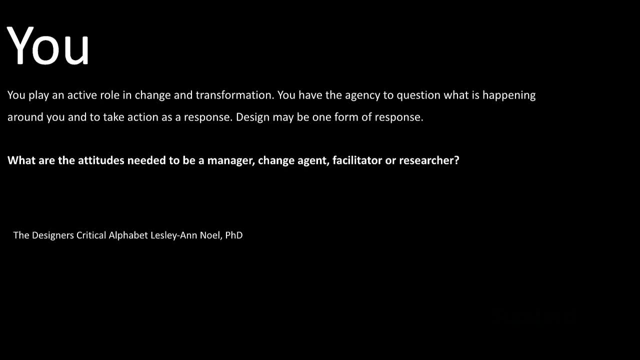 Unlearning oppression. What will you do to unlearn oppressive behaviors? You play an active role in change and transformation. You have the agency to question what is happening around you and take action as a response. Design may be one form of response. Question is: what are the? 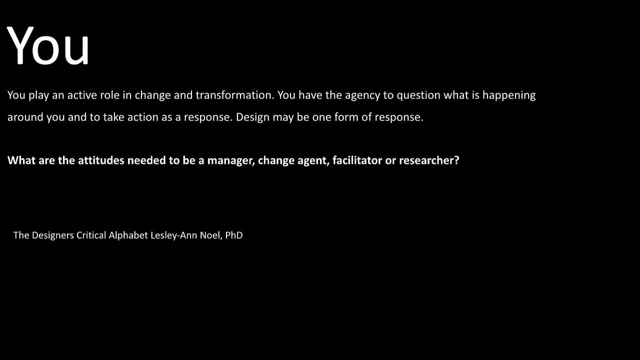 adults and adults involved. Who are they? They are the ones in the team. They are the ones who are called to act is what are the attitudes needed to be a manager, change agent, facilitator or researcher? This is a great set of cards here. 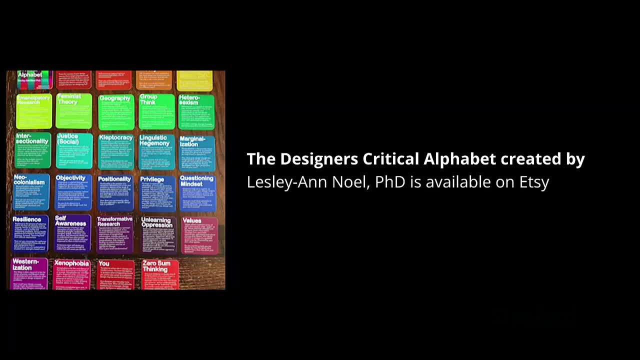 I have an image on the left-hand side of a set of cards from Dr Lesley-Ann Knoll called The Designer's Critical Alphabet. It is pretty amazing. I would recommend this for every designer to have in their toolkit. Have you tried VR? 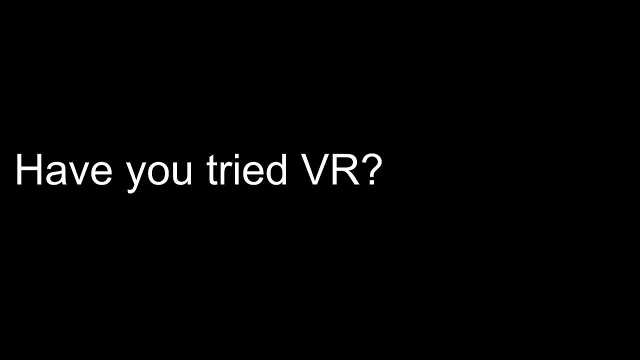 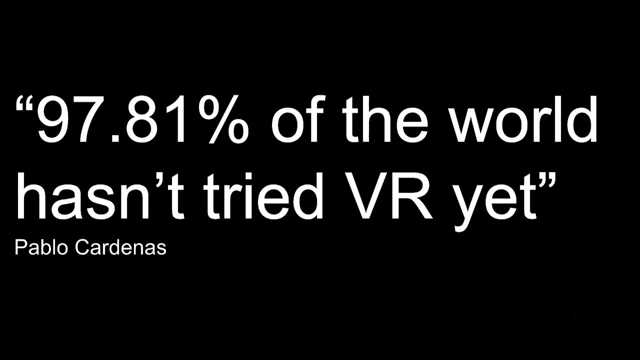 By a raise of hands. who has tried VR in the room? A majority of people in the room have tried VR. However, 97.81% of the world hasn't tried VR yet. Yes, A lot of people haven't tried it. 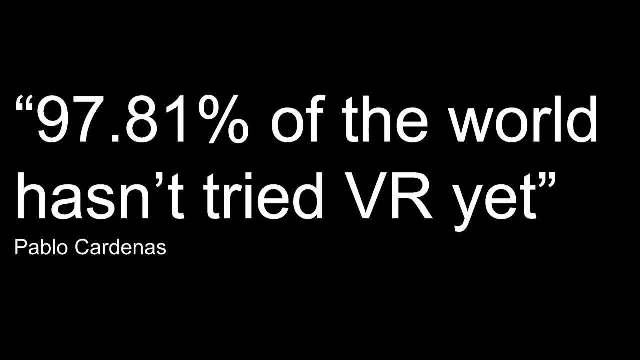 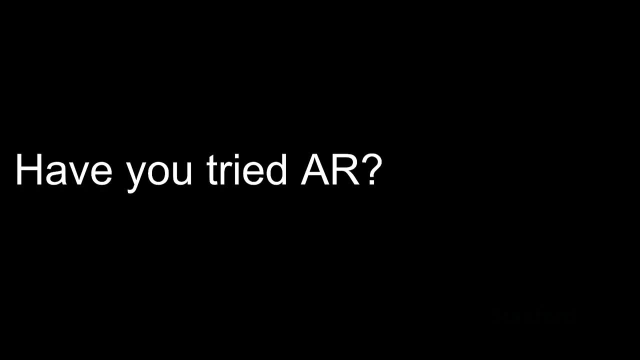 This is the truth And there are many reasons for that, so many reasons for this- But this is from Pablo Cardenas and he did a talk for A11y VR Meetup and talked about this in depth. Have you tried AR- augmented reality? 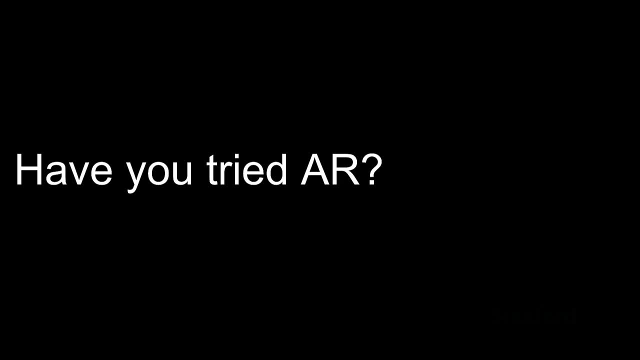 Has anybody tried AR? Sometimes people don't know they've tried AR because filters Anybody. ever use a filter for anything? Yes, Filters. Filters on your Instagram- Yep Bunch of you. So yeah, the truth is a lot more people have tried AR. 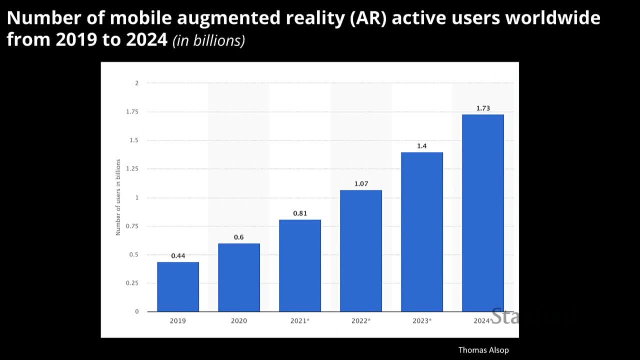 So here I have a chart of the number of mobile augmented reality active users worldwide from 2019 to 2024.. And these numbers are in billions. So in 2019, it was 0.44.. In 2020, 0.6.. 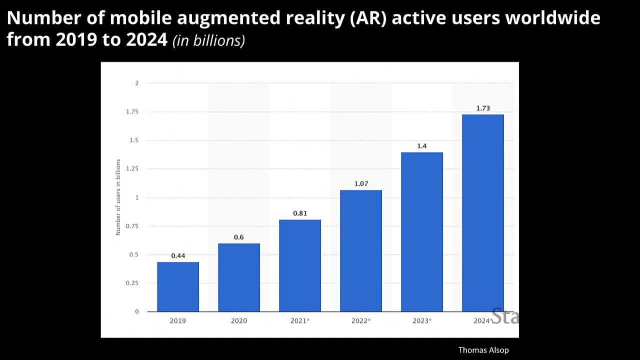 In 2021, 0.81. 0.8. 0.8. 0.8.. In 2022, is that the year we're in? I can't remember. This pandemic is messing me up. In 2022, 1.07 billion people. 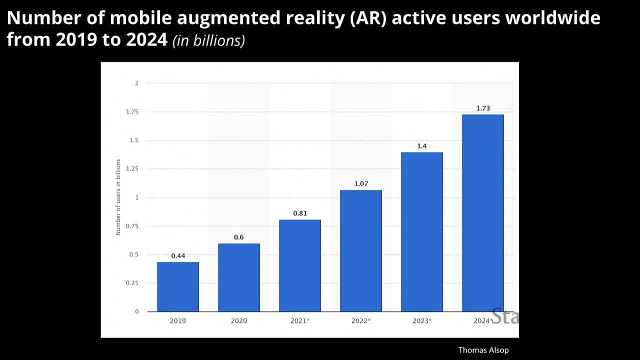 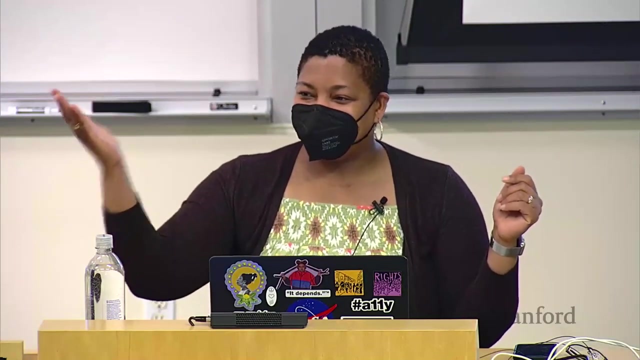 This is estimated in 2023, 1.4 billion And in 2024, 1.73 billion. How many people are in the world? Five plus six? Nobody knows. I think it's about, do you know? 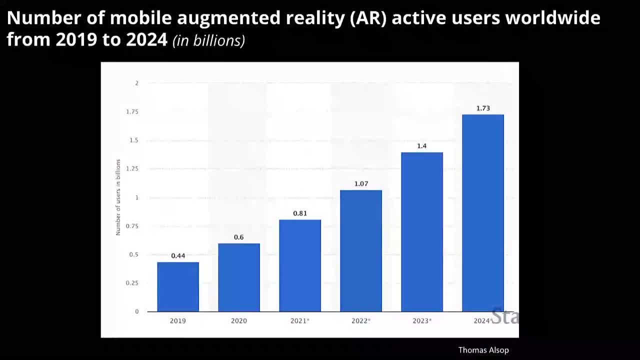 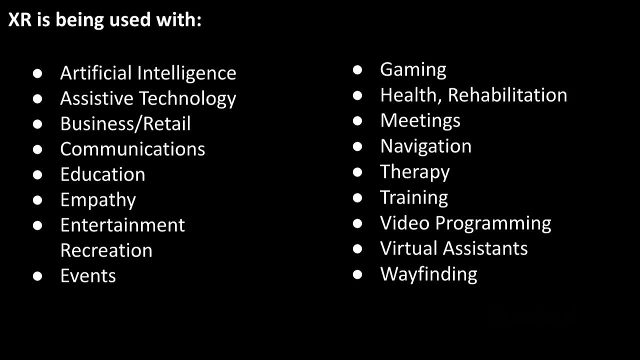 I think it is about 7 billion, So yeah, So currently XR is being used with artificial intelligence, assistive technology, business and retail communication, education, empathy, entertainment and recreation events, gaming- Yeah, Health and rehabilitation, meetings, navigation, therapy, training, video programming, virtual. 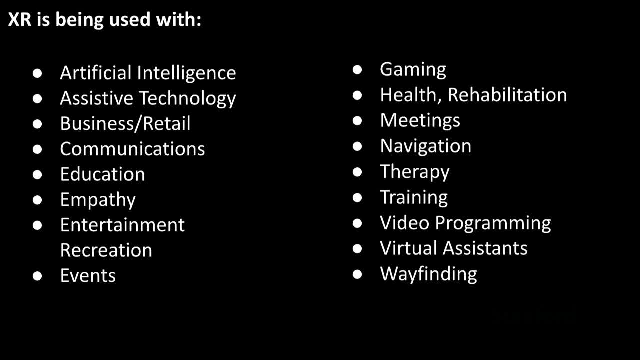 assistance and wayfinding. Does anybody use AR or VR for things other than entertainment in here? You do. We use VR for research. You use it for research. Okay, Yeah, So research and entertainment is what the room demographic is Okay. 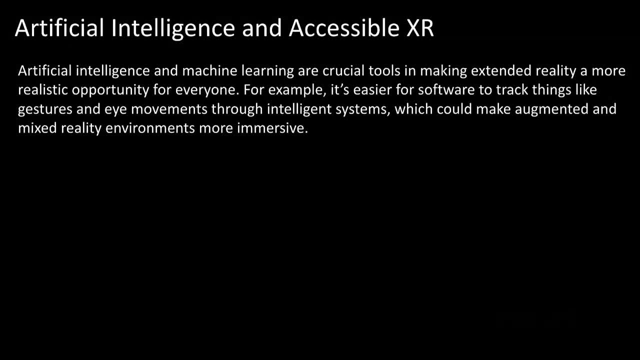 Cool, So I wanted to touch on artificial intelligence and accessible XR. So artificial intelligence and machine learning are crucial tools in making extended reality a more realistic opportunity for everyone. For example, it's easier for software to track things like gestures and eye movements through. 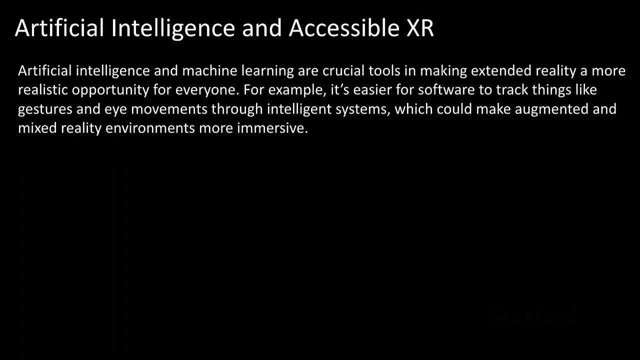 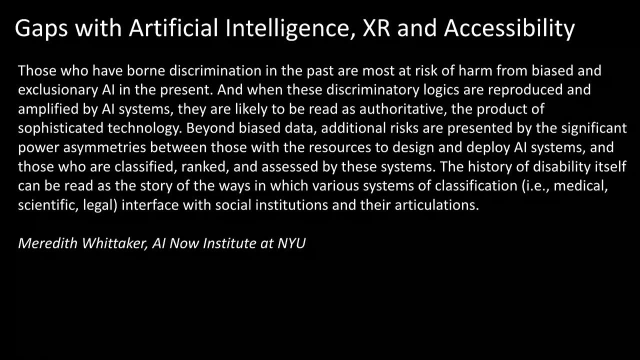 intelligent systems which could make augmented and mixed reality environments more immersive. Okay, Cool, Thank you. However, there are gaps with artificial intelligence, extended reality and accessibility. So those who have borne discrimination in the past are most at risk of harm from bias. 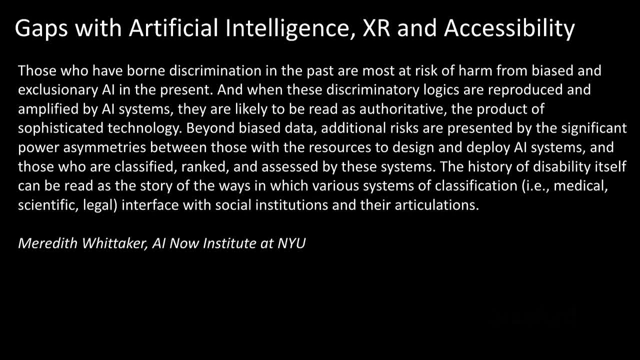 and exclusionary AI. in the present And when these discriminatory logics are reproduced and amplified by AI systems, they are likely to be read as authoritative The product of sophisticated technology. Beyond biased data, additional risks are presented by the significant power asymmetries between 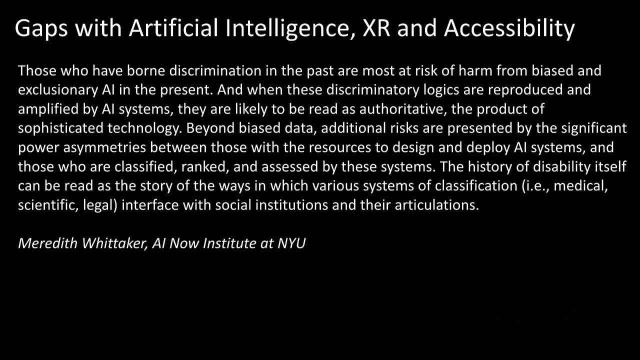 those with the resources to design and deploy AI systems and those who are classified, ranked and assessed by these systems. The history of disability itself can be read as a story of the ways in which various systems of classification, Ie medical, scientific, legal interface with social institutions and their articulations. 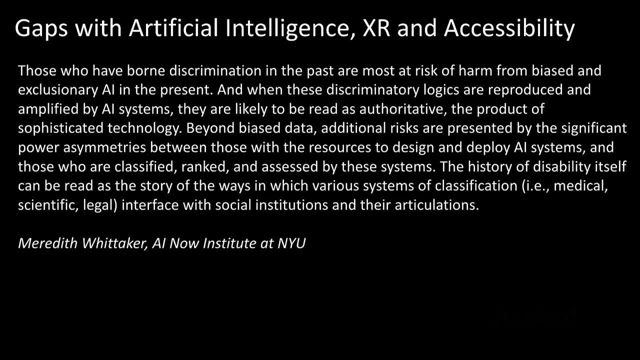 This is to say that AI oftentimes doesn't capture disability as it should, And if we're relying on this technology, you're either disabled or non-disabled, And if you're not disabled, you will be at some point, because that's life. 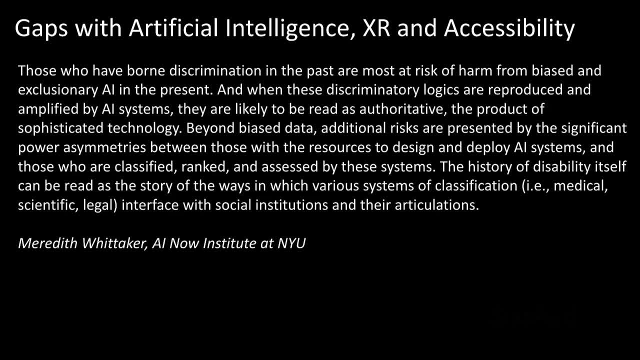 And if there's an AI that is determining your disability or not, I don't know if we really want that. So these are things that we have to get more informed about and get more involved with, Because we don't want AI totally determining everything for our lives. 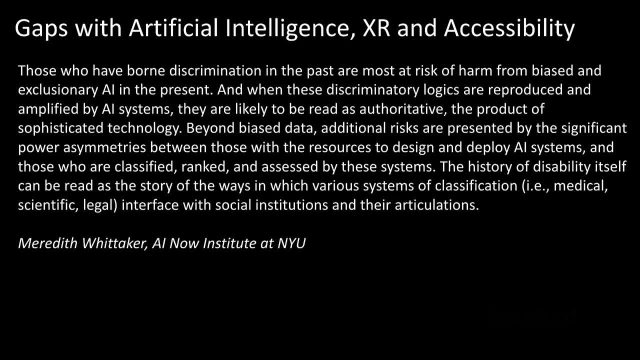 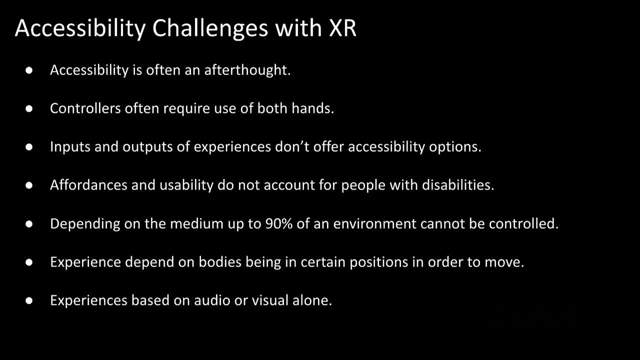 And this is from Meredith Whitaker and team at the AI Now Institute at NYU. So there are some accessibility challenges. with XR, Accessibility is often an afterthought. That's just straight up real. How many of you make stuff in here? How many of you incorporate accessibility? 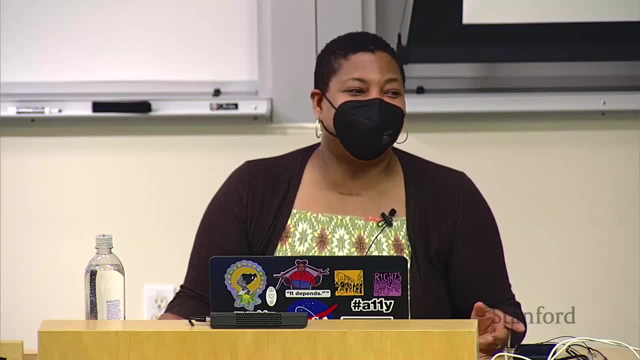 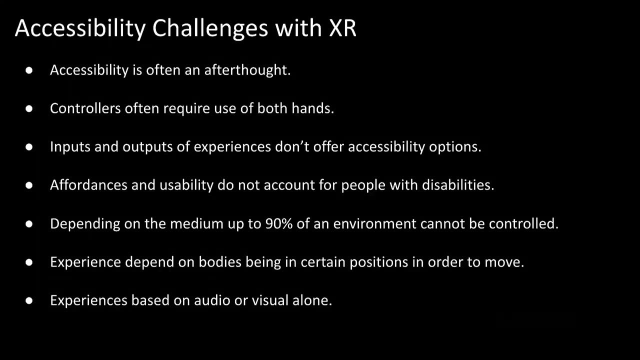 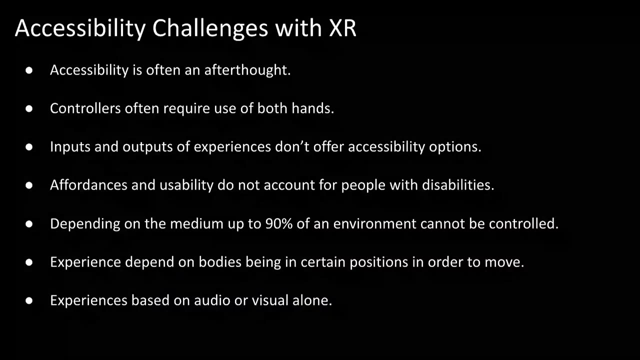 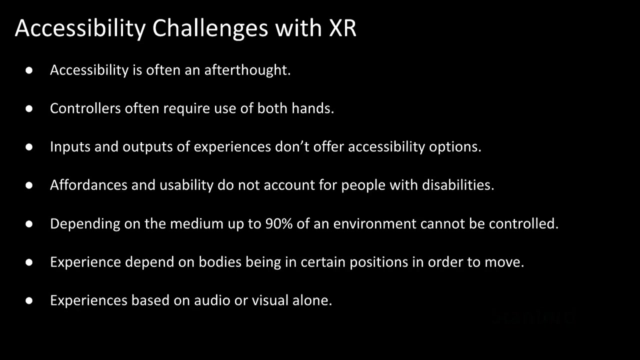 Be honest, It's an afterthought or not a thought. So some of the challenges with XR is that controllers require both hands. Experiences and outputs of experiences don't offer accessibility options. Affordances and usability do not account for people with disabilities. 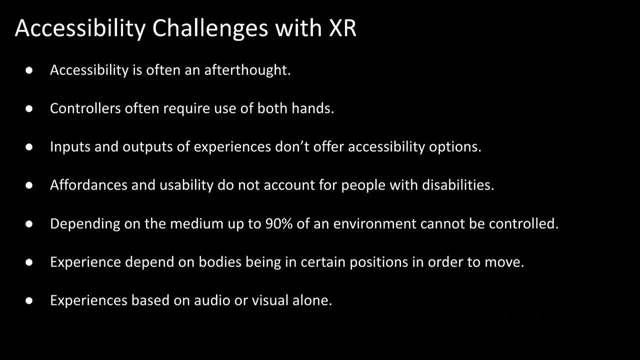 Depending on the medium, and this is especially with AR, 90% of an environment cannot be controlled. Experience depends on bodies being in a certain position in order to move, And experiences are based on audio or visual alone. Okay, So the W3C has some guidance. 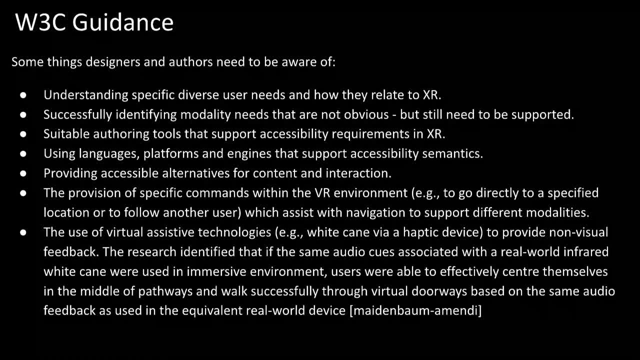 Some things designers and authors need to be aware of: Understanding specific, diverse user needs and how they relate to XR. Successfully identifying modality needs that are not obvious but still need to be supported. Suitable authoring tools that support accessibility requirements. Do I have any developers in the house? 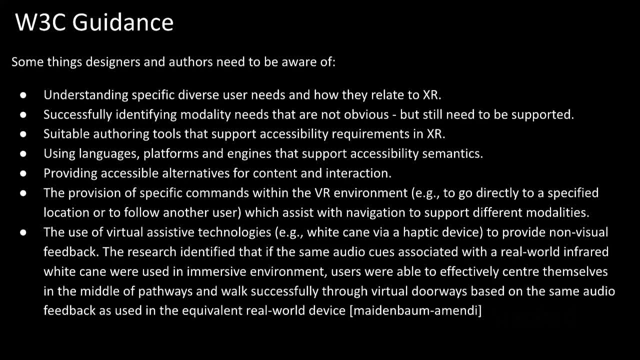 None. Okay, I'm going to bore some people. I'll just maybe go through it and I can send you the slides. Using languages, platforms and engines that support accessibility. semantics Providing accessible alternatives for content and interaction. The provisions of specific commands within the VR environment. 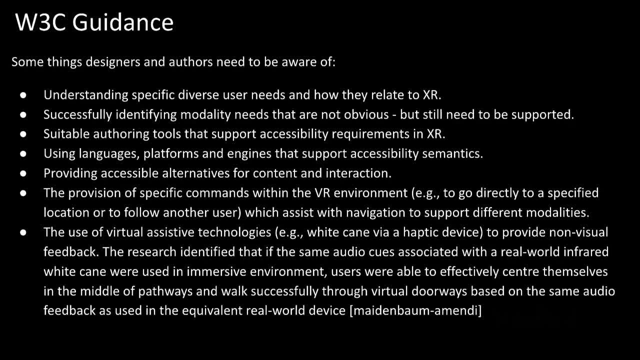 So, for example, to go directly to a specified location Or to follow another user. Okay, You can use a virtual assistant user which assists the navigation to support different modalities And the use of virtual assistive technologies, For example white cane. 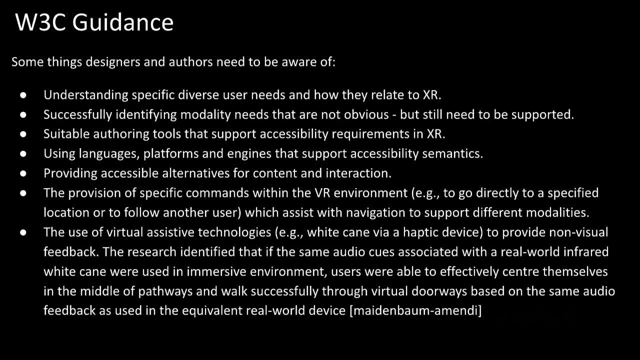 Via a haptic device to provide non visual feedback. So the research identified that if the same audio cues associated with real world infrared white cane were used in an immersive environment, users were able to effectively center themselves in the middle of pathways And walk successfully through the environment. 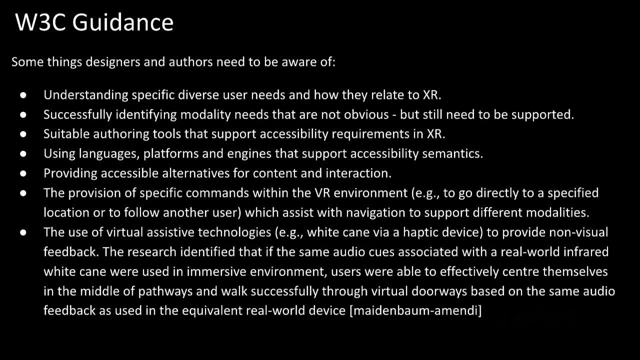 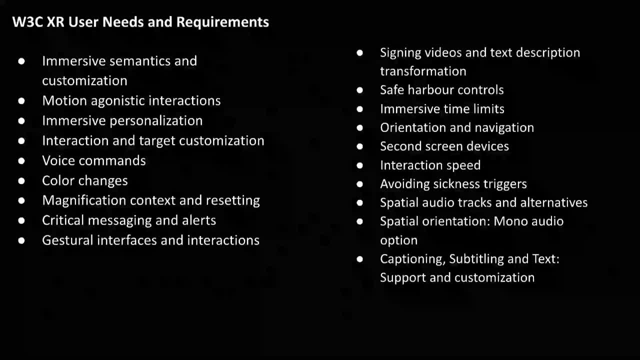 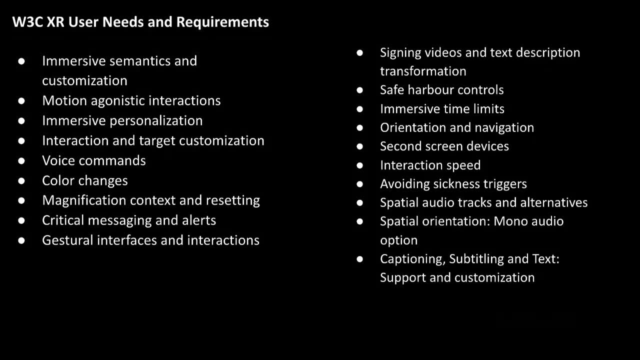 Okay, Successfully- through virtual doorways based on the same audio feedback as used in the equivalent real-world device. So here are some of the w3 people here familiar with w3c? No, Okay, so I'll just. I'll just start this. W3c is a world wide web consortium. 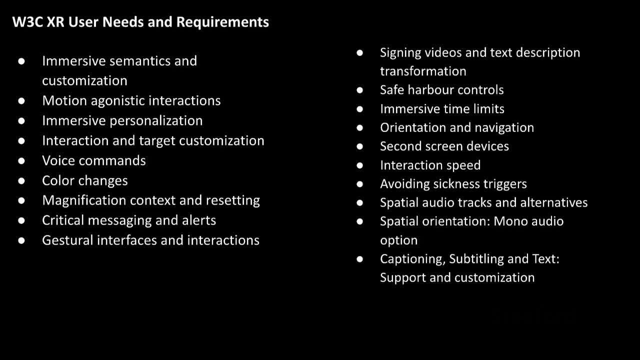 everybody who works on the web should know about the w3c. if You do anything web related, you should know about the w3c. go google them. They are Not. they are the international standard. they have put forth the web content accessibility guidelines and Such. they have also put out some XR user needs and requirements. 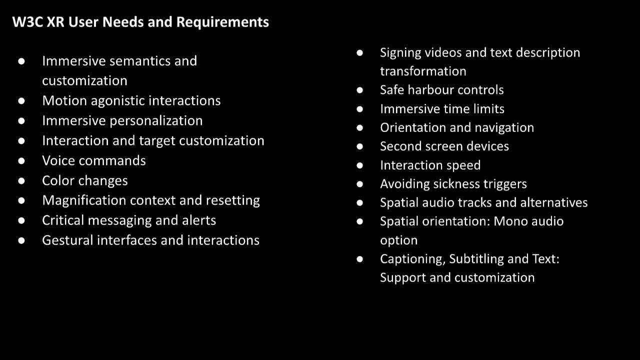 So I'm going to go over some of those. So here are some of the the XR user needs and requirements: immersive semantics and customization. motion agnostic interactions. immersive personalization interaction and target customization. voice commands, color changes, magnification, context and resetting critical messaging and alerts. gestural interfaces and interactions. 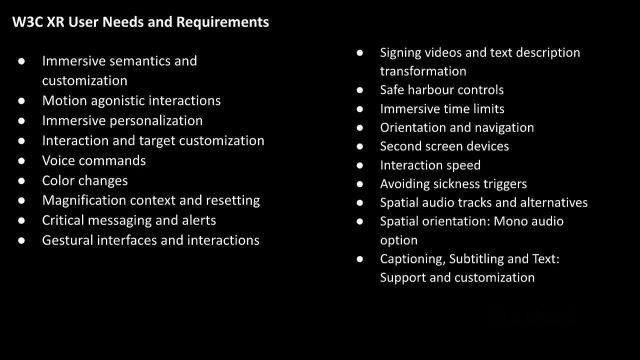 Signing videos and text description, transformation, safe Harbor controls, immersive time limits, orientation and navigation, second screen devices, interaction speed, avoiding sickness triggers, spatial audio tracks and alternatives, spatial orientation, mono-audio option, captioning, subtitling and text, with support and customization. Why is accessibility and XR important? 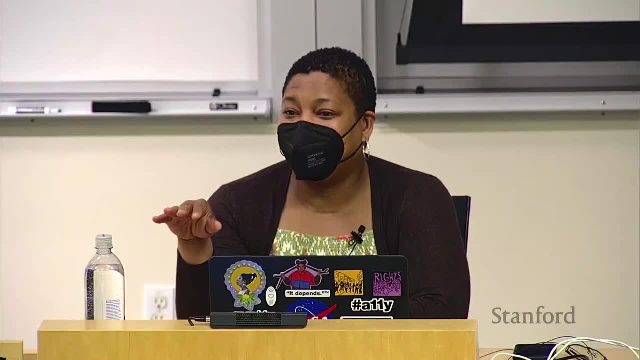 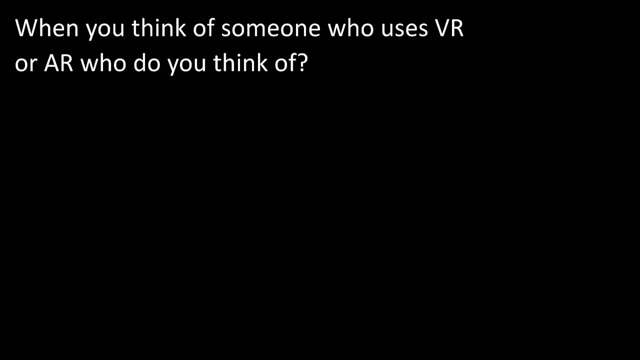 It's the right thing to do. Period, it really is. So I'm gonna ask the people in this room to answer me. if you're paying attention. When you think of someone who uses VR or AR, who do you think of? Can you please describe them to me? 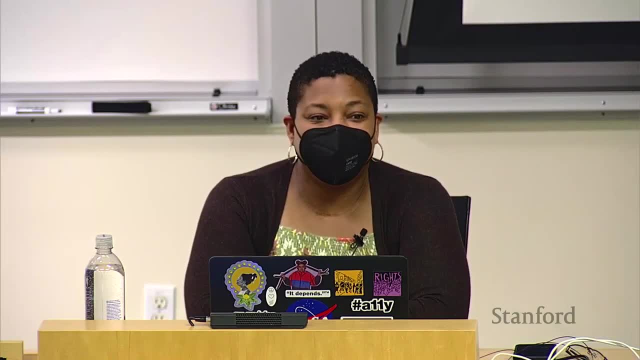 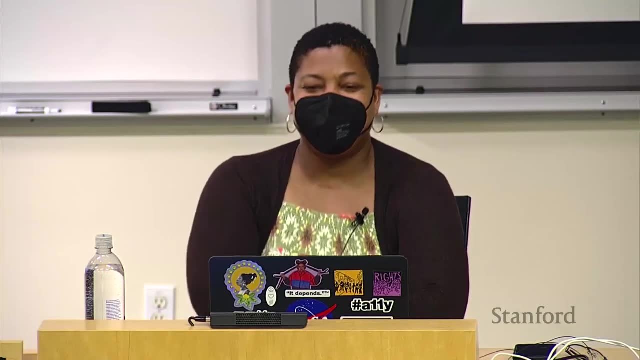 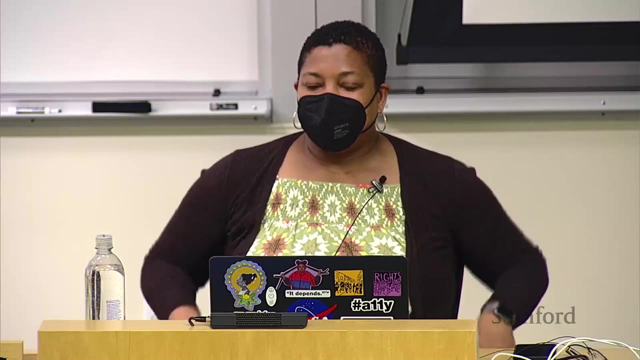 Can you please describe them to me? I will call on people. Thank you, I think of someone because I'm not. I think of someone who's young and active and very tech savvy. I think of someone because I'm not. I think of someone who's young and active and very tech savvy. 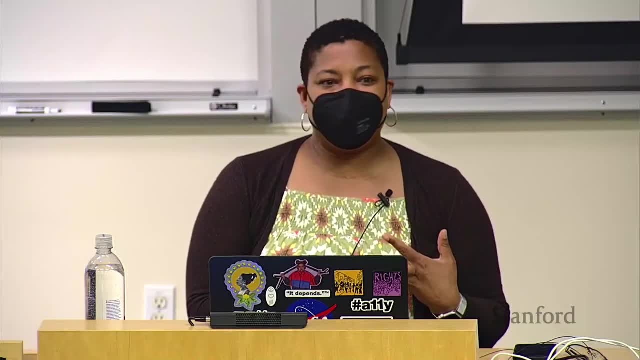 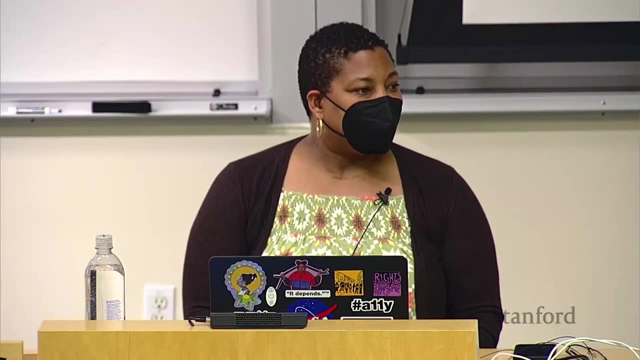 Somebody who is young and active and tech savvy: Okay, Anyone else? Yes, I think of those videos of like this 25 year old guy, guy like walking around a room, like bumping into things, you know like the kind of like, um, stereotypical, like six foot tall white male: okay, so a six foot tall 25 year old white male? 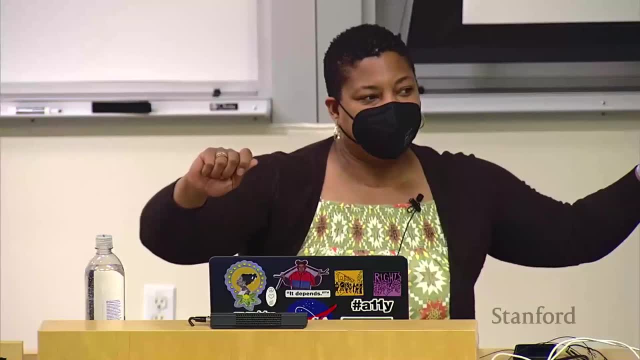 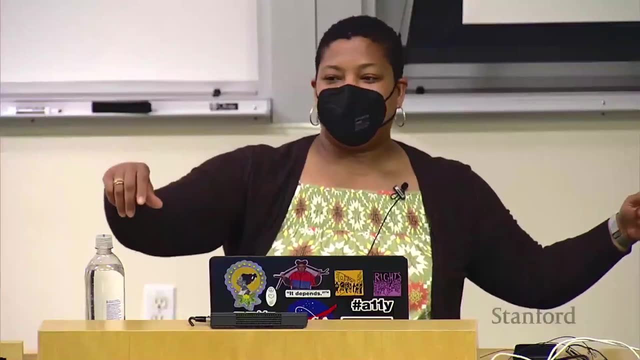 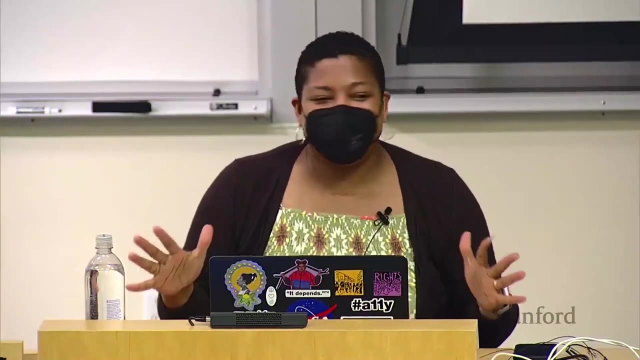 who's in a big enough space to like walk around and bump into things. that's who you're picturing for vr. anyone else picturing that person? yeah, kind of mark zuckerberg, but in that space, okay, mark zuckerberg type. yeah, yes, i'm picturing basically that, but 14 years old. 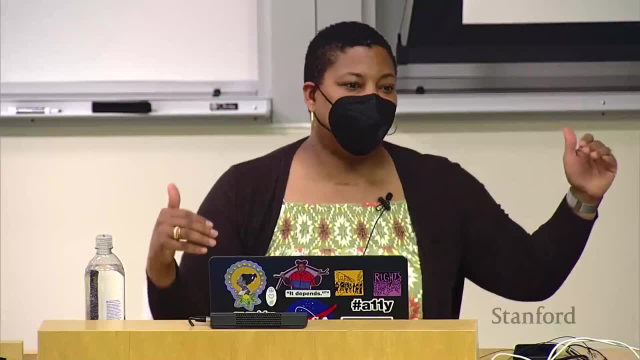 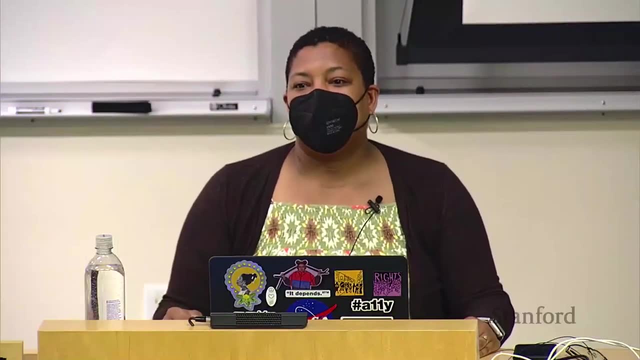 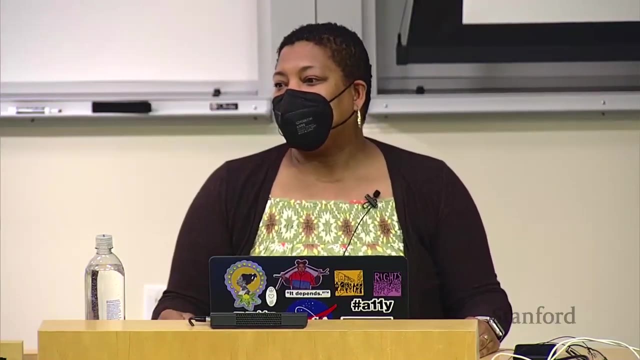 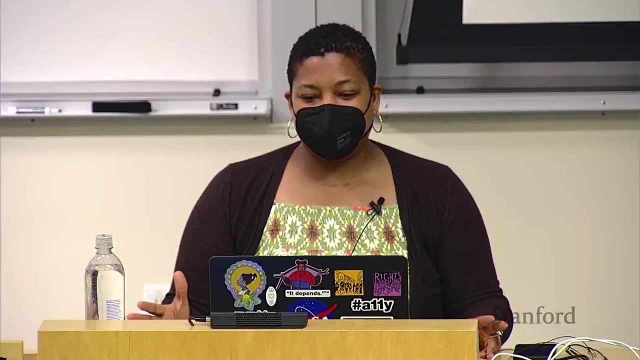 okay, so 14 year old, who's maybe not as six feet tall, but also white male? yes, okay. yes, back here. i think maybe some like anti-social people, some anti-social people. okay, gamer types: what's a gamer type? i mean like someone who likes video games, somebody anybody who likes video games. okay, yeah, so this is very. 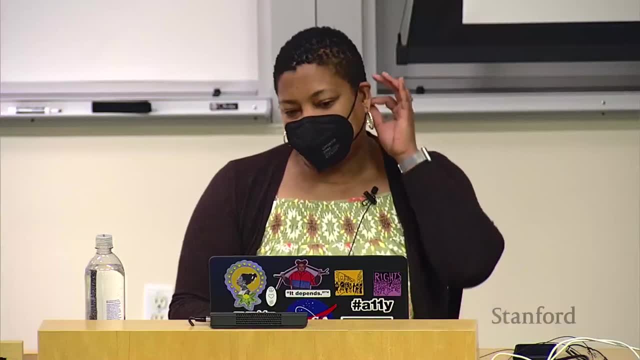 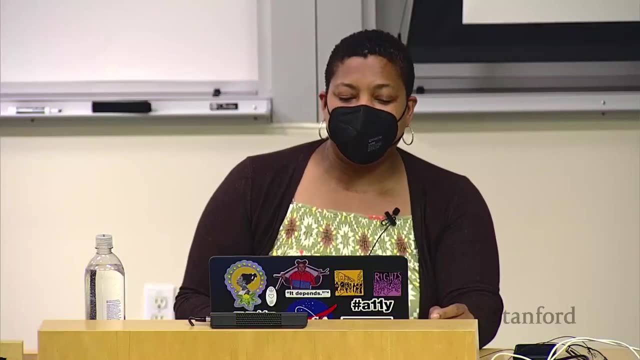 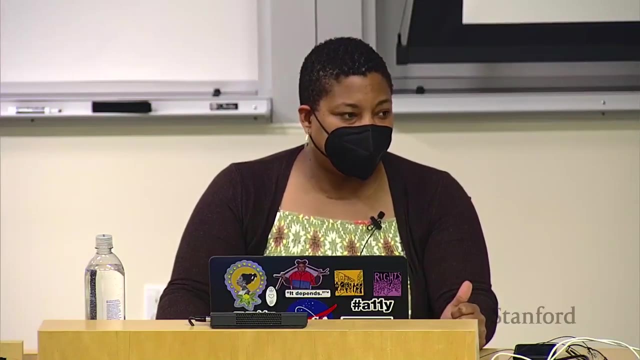 interesting to me because, uh, just a few weeks ago i was working with my grad research assistants and i asked those questions. you know, designers focus on human-centered design, but which humans are we actually focusing on? are we focusing on the non-binary person who is 45 years old? 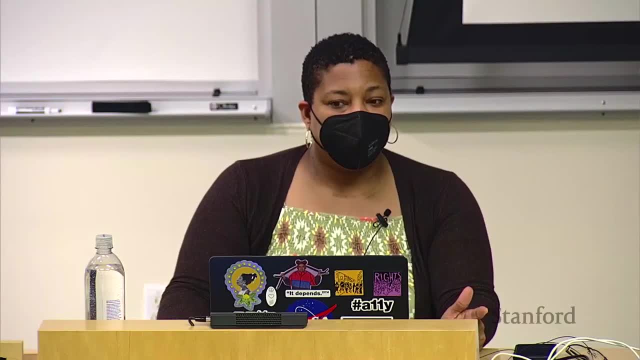 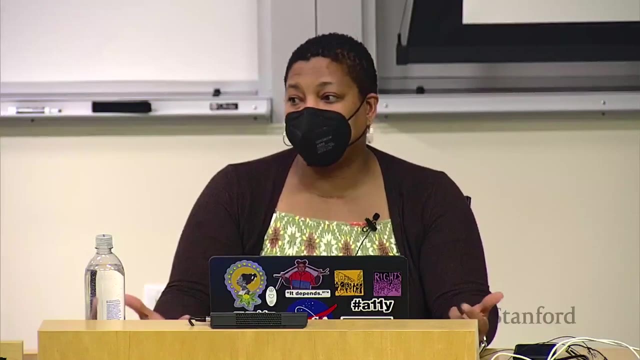 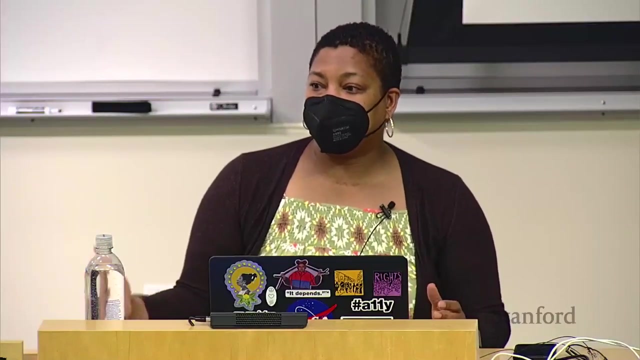 in a wheelchair, who's uh has low vision? the answer is no. and why aren't we? is the question i'm asking to you all as creators, designers, developers. which humans are we actually focusing on, and does the focus need to continually be the 25 year old or the 14 year old white guy? because that's what we're focusing on. 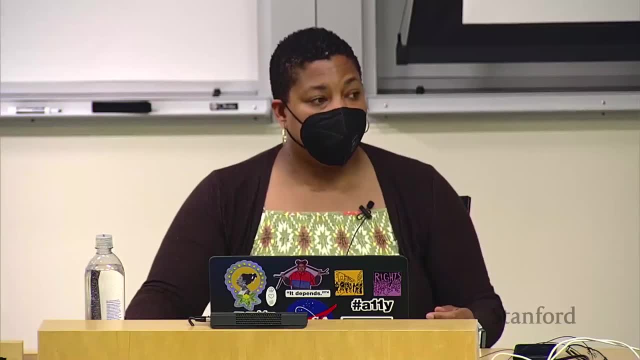 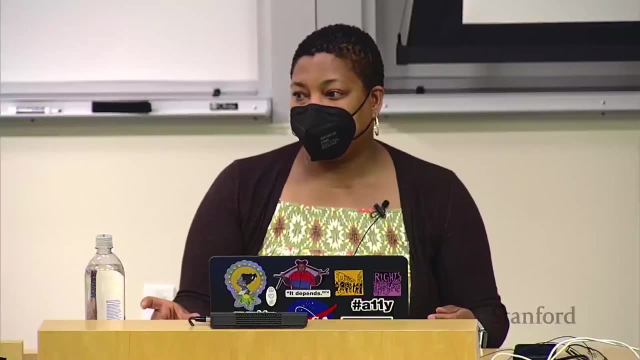 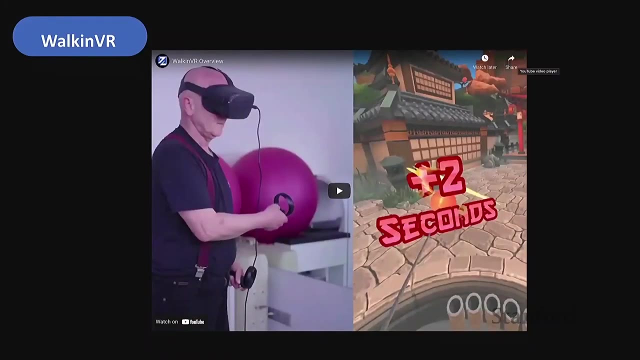 what we we we think about when we think about a gamer, and we need to flip that and really start to think about the real humans that actually use the stuff we produce. so i have a video and i didn't practice this. i hope this video goes, but i want to introduce you all to walk in vr, which is a 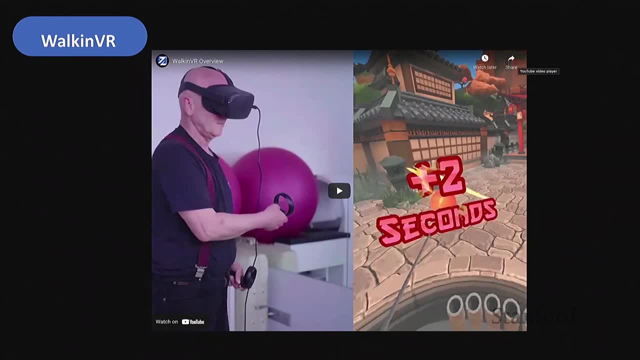 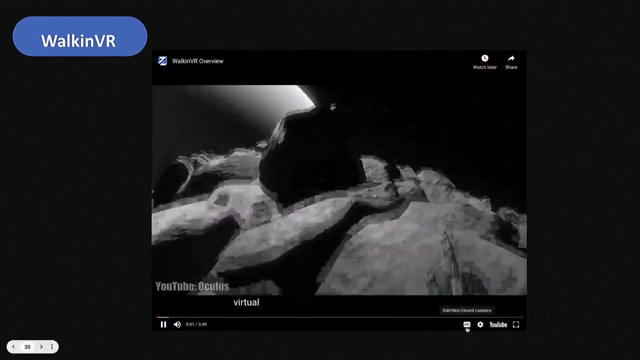 it's a cool thing. i'll talk about a little bit after, but this video runs about three and a half minutes. will the sound go through? okay? let's just hope this doesn't blast people away. it's too loud. wait, it's gone. it could be an amazing thing. it gives people the opportunity to experience things. 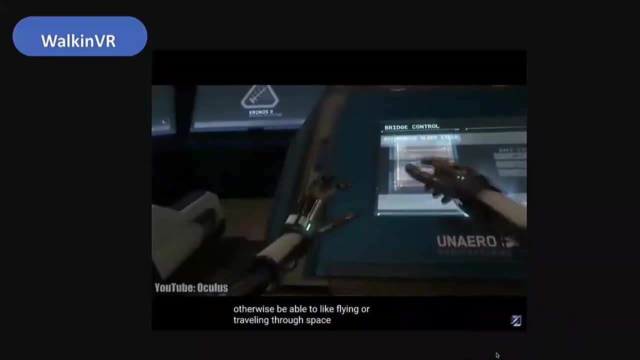 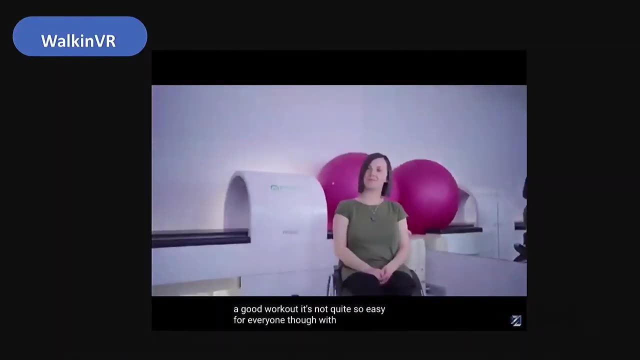 they wouldn't otherwise be able to like flying or traveling through space, as well as more down to earth activities such as getting a good workout. it's not quite so easy for everyone, though. with virtual reality or vr, you use real world movements to control your actions in the virtual. 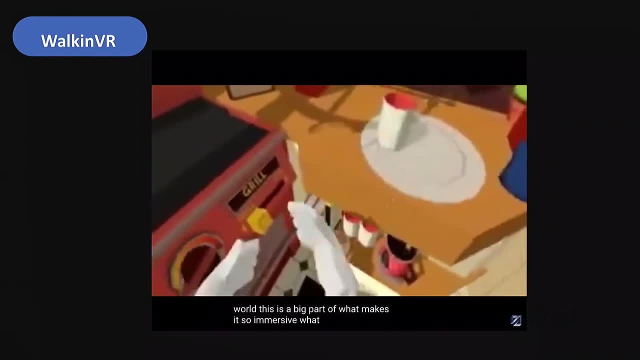 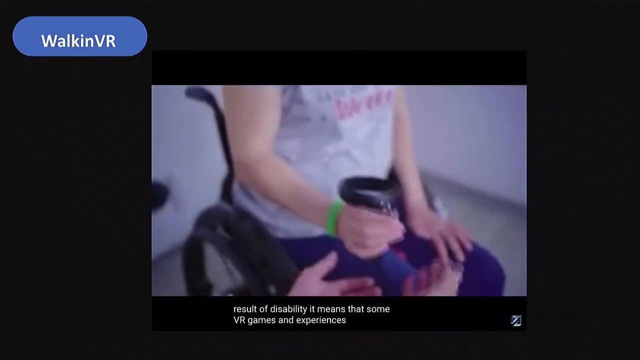 world. this is a big part of what makes it so immersive. what happens when your real world movements are limited as a result of disability? it means that some vr games and experiences simply not an option for you. for example, a game may require you to turn around, but if you use a, 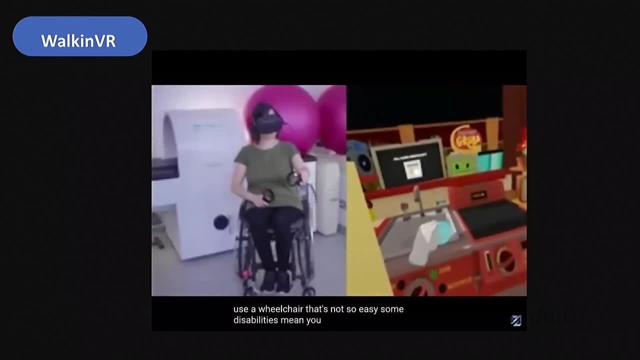 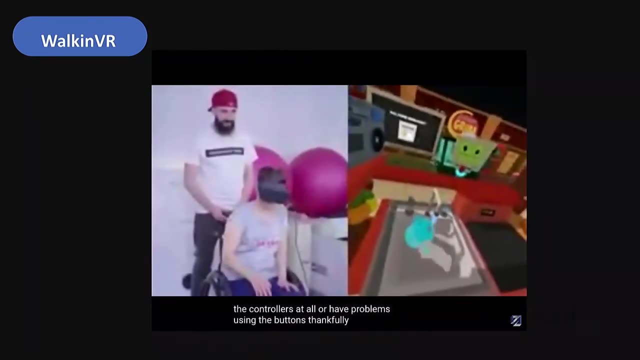 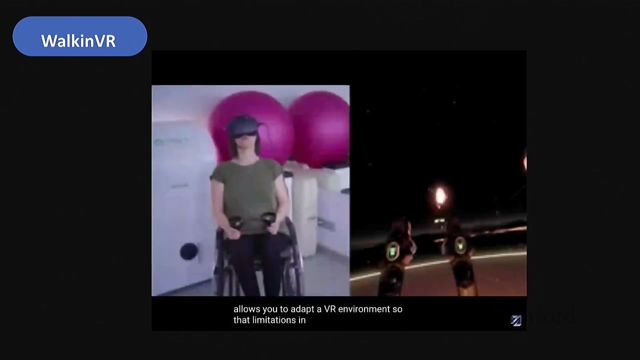 wheelchair, that's not so easy. some disabilities mean you can't grip things firmly, so you may not be able to hold the controllers at all or have problems using the buttons. thankfully, there's a solution. walking vr is software that allows you to adapt the vr environment so that limitations in your movement don't have to mean. 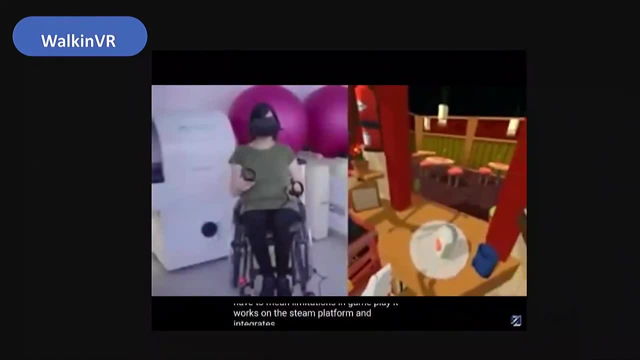 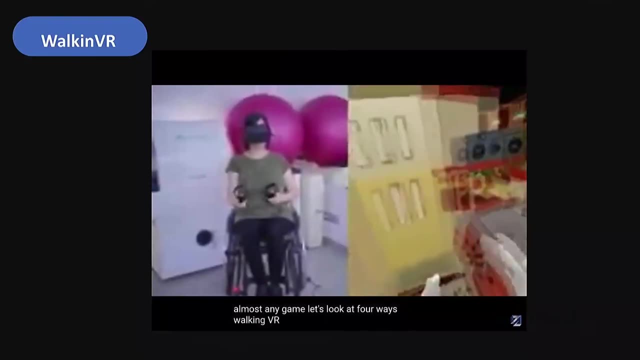 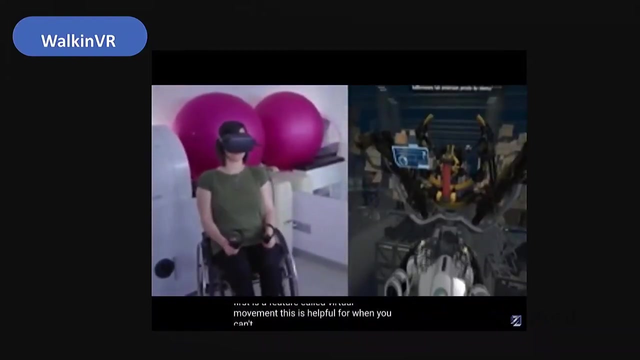 limitations in gameplay. it works on the steam platform and integrates with the steam vr environment, meaning it can be used successfully with almost any game. let's look at four ways walking vr can adapt virtual reality. the first is a feature called virtual movement. this is helpful for when you can't walk. 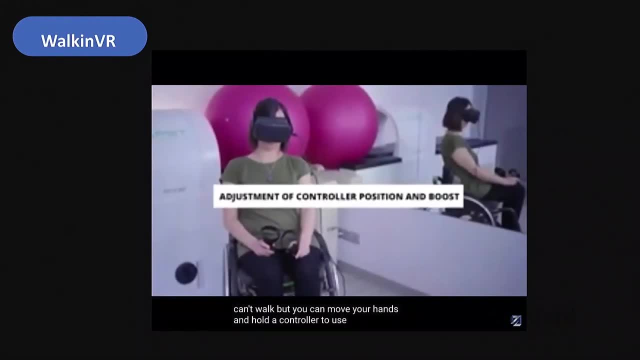 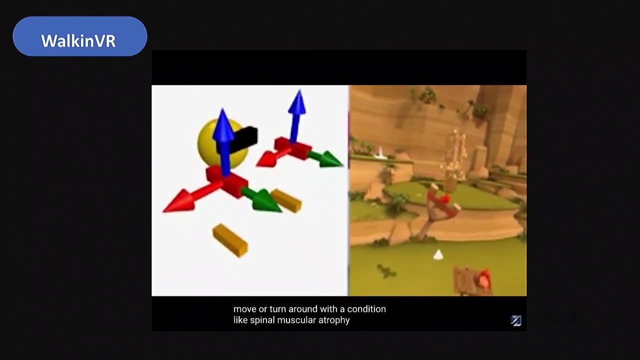 but you can move your hands and hold a controller. to use it, you simply grab space with a button and then move or turn around. with a condition like spinal muscular atrophy, you might be able to hold the controllers but not maintain them at the height required by the game. in this situation, 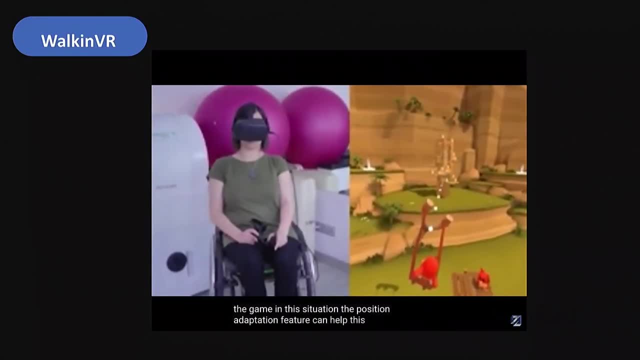 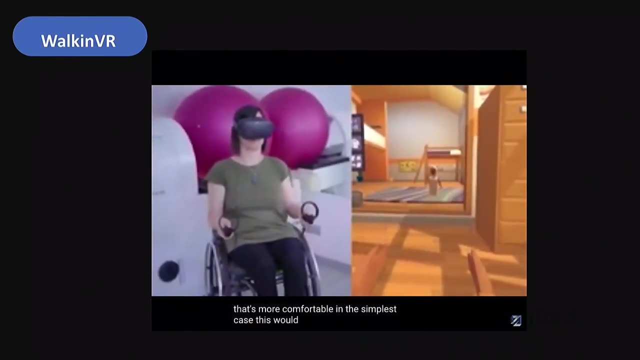 the position adaptation feature can help. this allows you to adjust the position in which the controller needs to be held to one that's more comfortable. in the simplest case, this would mean changing the height, but there are more ways to adjust the position in which the controller needs. 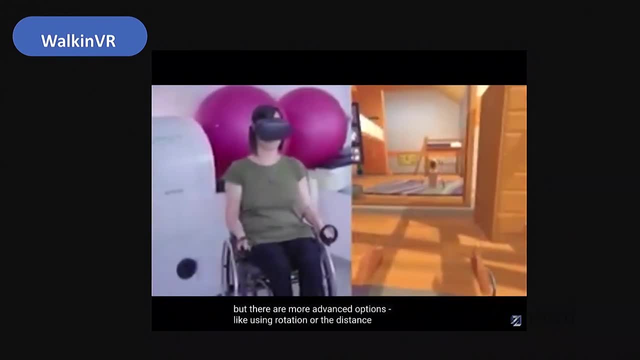 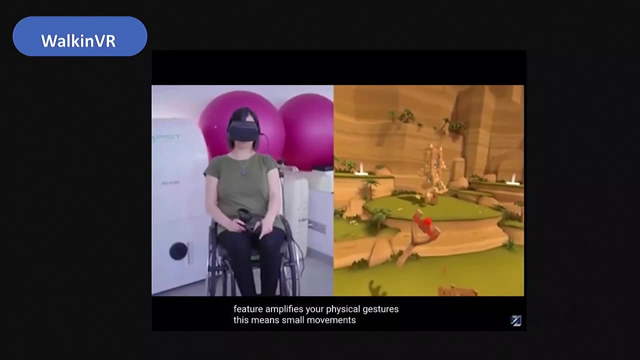 to move like you sign up with your camera and charms, and you also need to adjust the position to move more by cams. in addition to some of the more advanced options too, like using rotation or the distance the controller is from your body, the boost feature amplifies your physical gestures. this 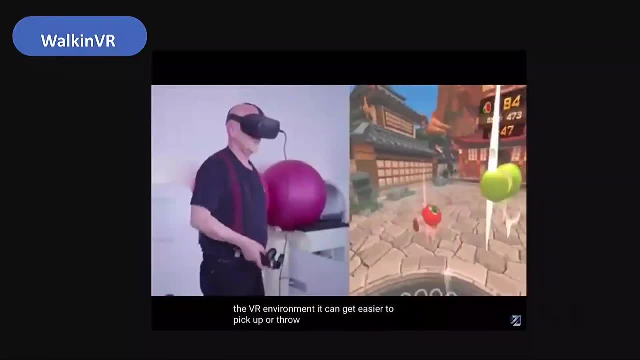 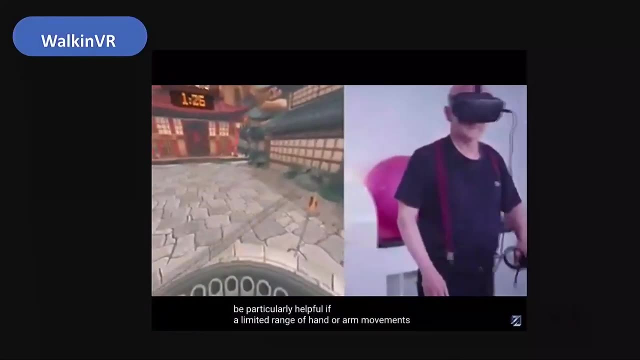 means small movements in the real world translate to much larger ones in the vr environment. it can get easier to pick up or throw virtual items. this can be particularly helpful if you have a limited range of hand or arm movements. another feature is the ability to set different parameters for each. 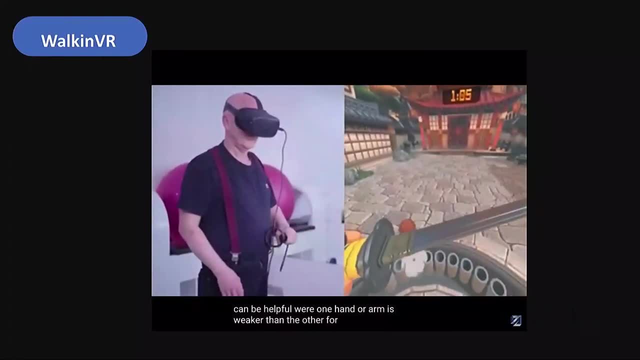 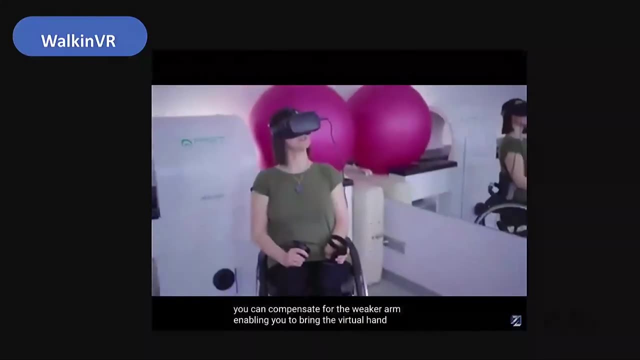 this can be helpful where one hand or arm is weaker than the other. for those that have had a stroke, say, this feature means you can compensate for the weaker arm, enabling you to bring the virtual hand up into your field of vision, something that can have a positive psychological effect. 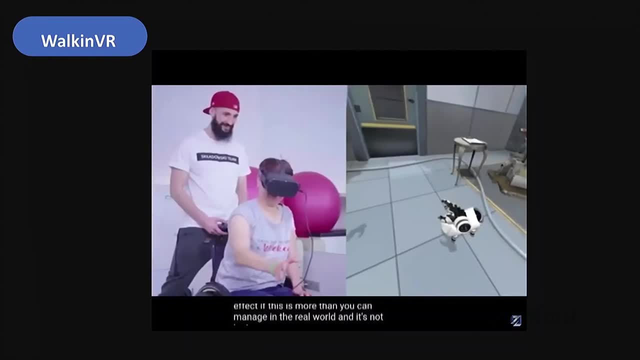 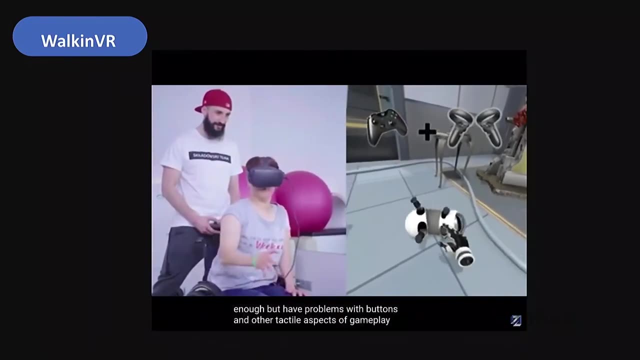 if this is more than you can manage in the real world- and it's not just a position- you can adjust. some people can move the controllers well enough, but have problems with buttons and other tactile aspects of gameplay. for these people, there is the personal assistant function. this allows another. 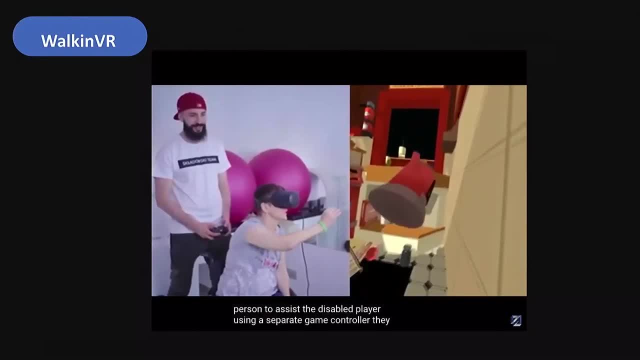 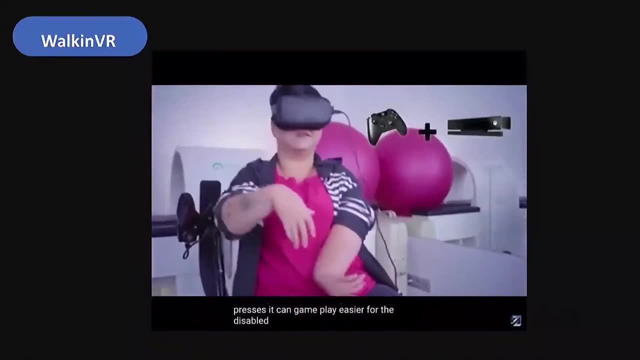 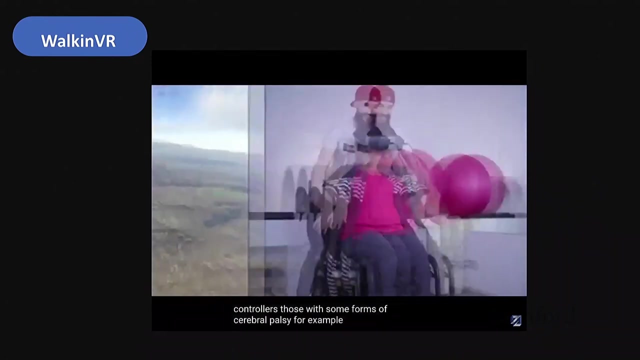 person to assist the disabled player using a separate game controller. they can make helpful adjustments to the avatar's position and also perform button presses, making gameplay easier for the disabled user. there's also a large group of people who have problems holding controllers: those with some forms of cerebral palsy, for example, attaching the controllers to yourself. 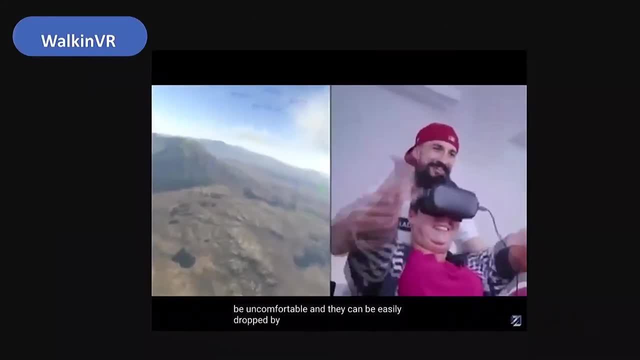 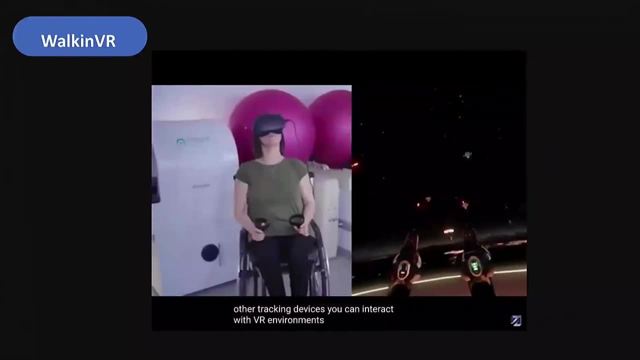 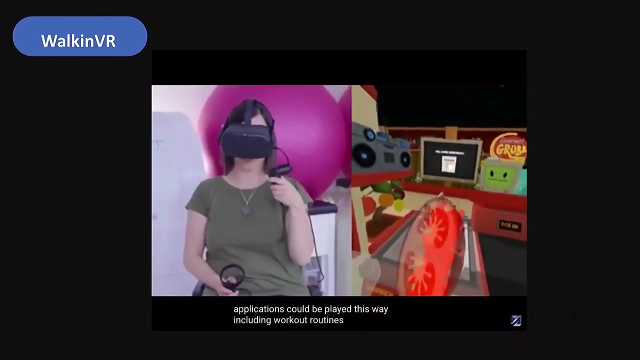 in some way can be uncomfortable and they can be easily dropped. by using walk-in vr in conjunction with connect and potentially, other tracking devices, you can interact with vr environments without the need for a controller. indeed, many games and applications can be played this way, including workout routines. put together, all these features mean you can. 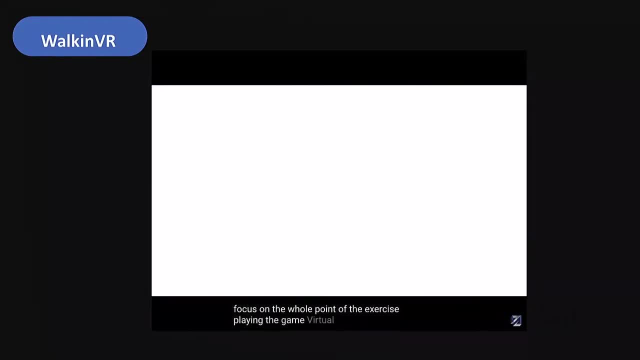 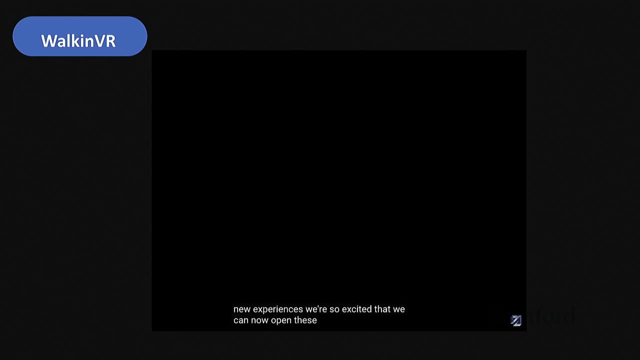 finally, focus on the whole point of the exercise: playing the game. virtual reality offers a great way to have fun, workout and try new experiences. we're so excited that we can now open these possibilities up to a wide range of people. and we can now open these possibilities up to a wide 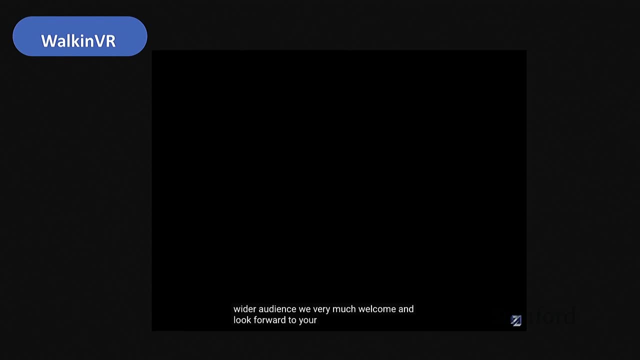 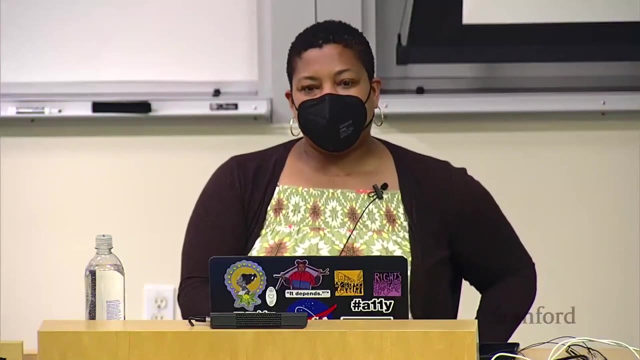 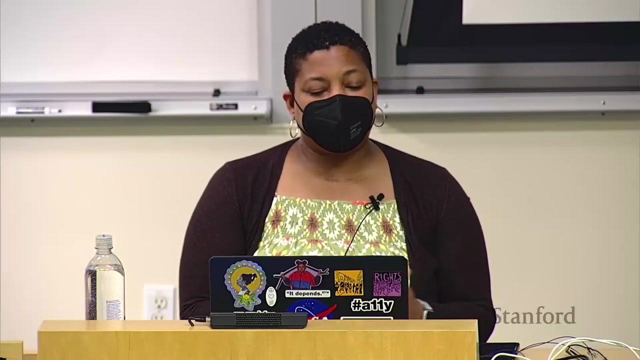 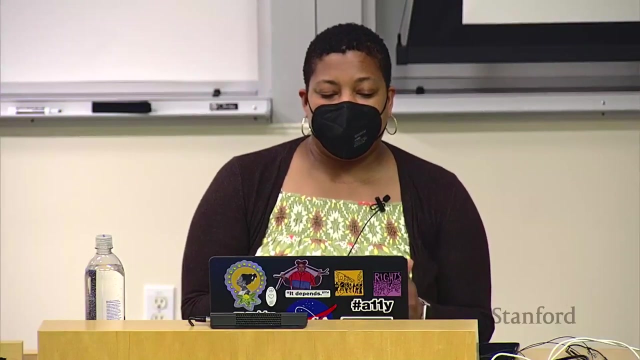 audience. we very much welcome and look forward to your comments and feedback. so walk-in vr is available on steam and it's adapting vr games for people with disabilities. walk-in vr has been tested to make vr accessible for people with cerebral palsy, spinal cord injury, traumatic brain injury, muscular dystrophies, spinal muscular atrophy. 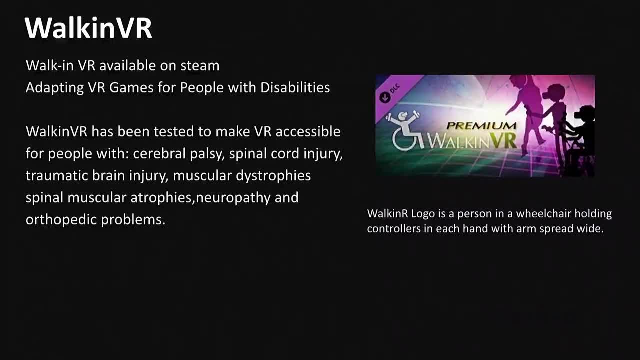 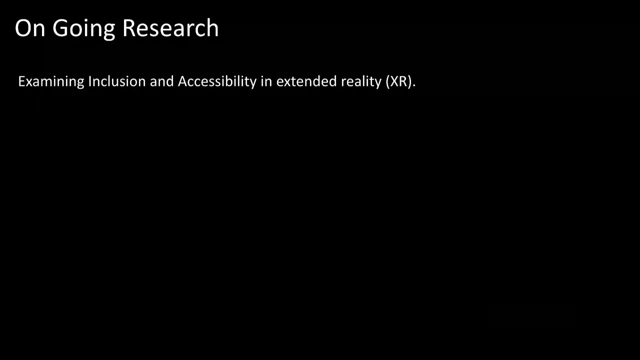 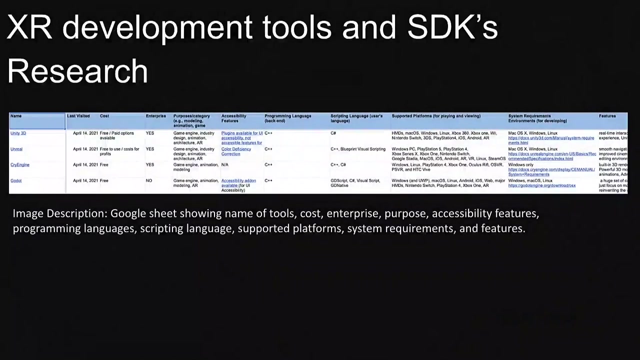 neuropathy and orthopedic problems. on the right i have a an image of the walk-in vr logo is a person in a wheelchair holding controllers in each hand with arms spread wide. so this is my ongoing research. i'm examining inclusion and accessibility in the extended reality space, um, one of the first. 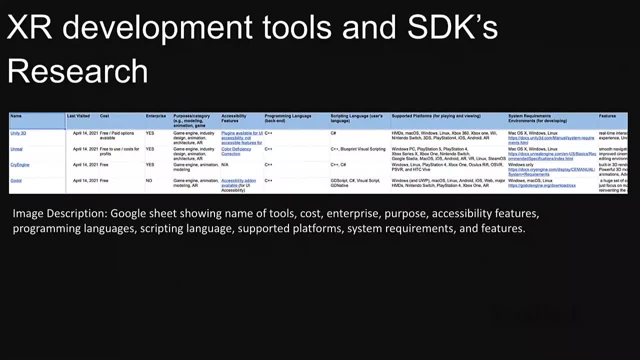 things i started with. uh, here i have an image of a google sheet showing names of people with cerebral palsy and i have an image of the first person or a group of people with cerebral palsy on the social media. so i have the field names of tools, cost, enterprise, purpose, accessibility, features, programming. 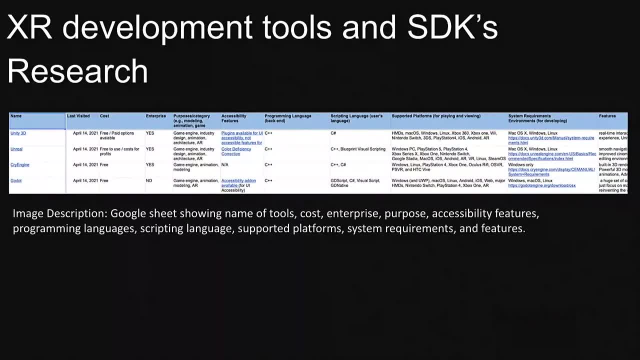 languages, scripting languages, supported platforms, system requirements and features. so when i first said i'm gonna research inclusion and accessibility, i didn't know what i was thinking. first of all, that's huge right. so i said where should i start? and i decided to start with the tools. the tools. 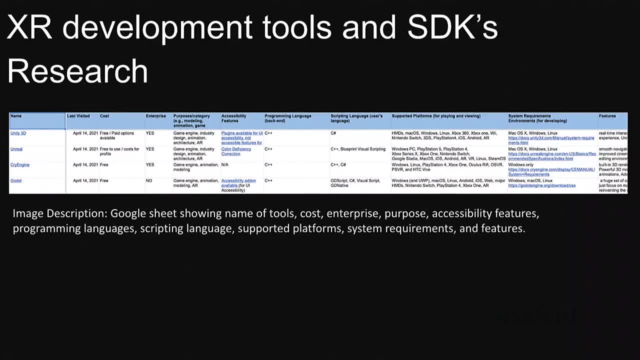 that are used to create experiences started looking at. do the tools cost money? Do they have certain system requirements? Do they require a certain level of knowledge from someone in order to participate? So, do I have any Unity users in here? Yes, a little bit. So for those who don't know Unity, Unity is created to make games. 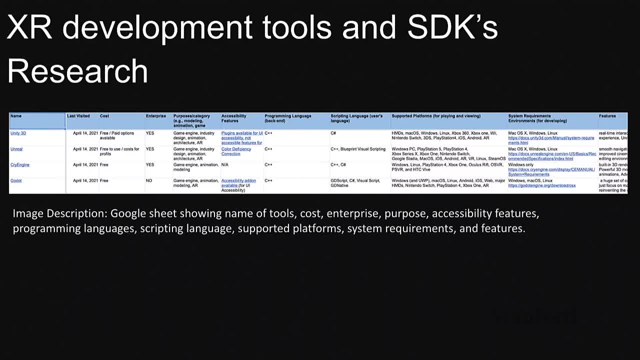 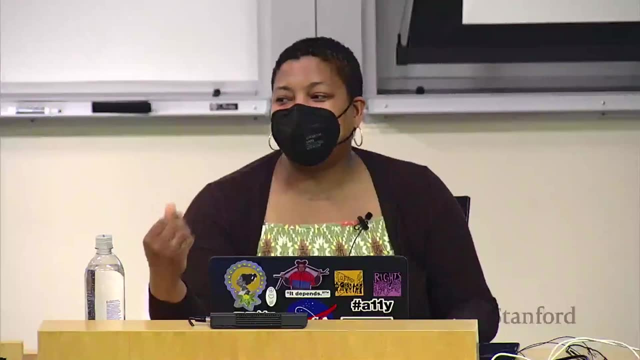 It's also created to make a lot of virtual reality experiences, And it's really helpful if you know C Sharp, Because if you are using Unity hands down, you are going to change a script at some point And if you don't know C Sharp, you're going to have some trouble. 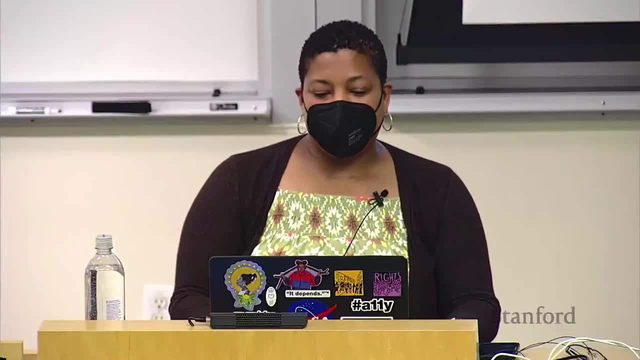 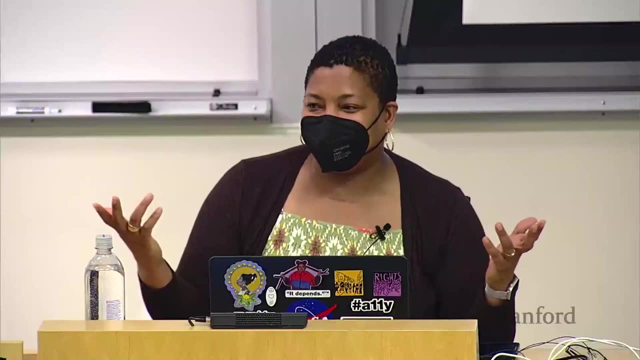 And that's a barrier to entry, right. So, you know, I was like this is boring, Like who wants to see this spreadsheet? Nobody wants to look at the. I mean, would you all? I mean, right, Like nobody's looking at this thing. So I, working with Saki Asakawa, 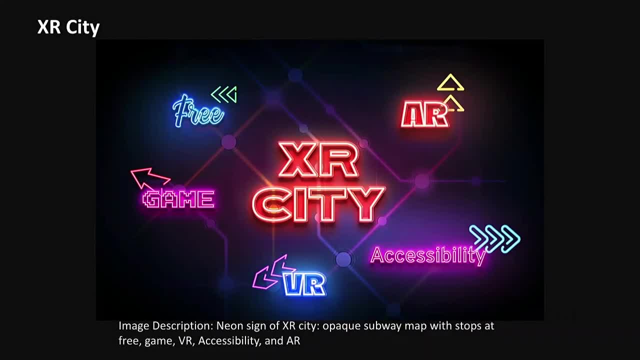 we came up with XR City, right? So you want to learn about XR, but you don't know how. So what do you need? A map, right? So here the image is of a neon sign of XR City. There's an opaque subway map. 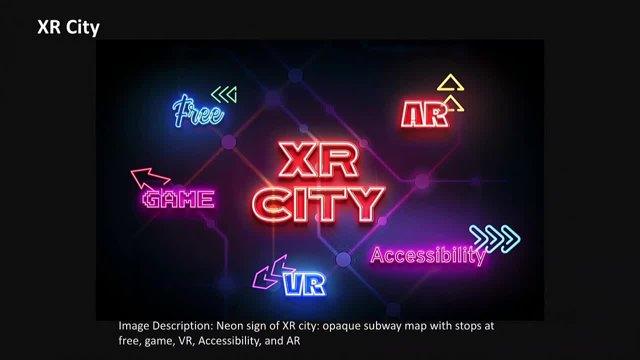 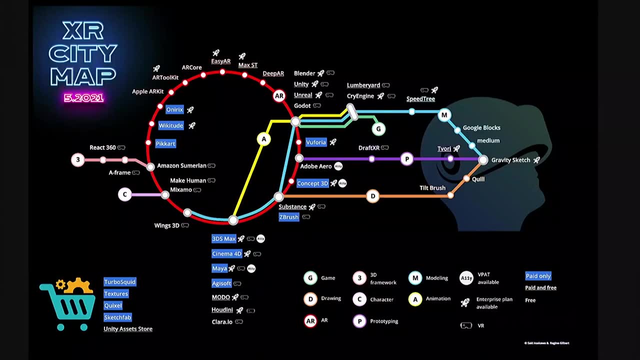 with stops at free game, VR, accessibility and AR. So this is what we came up with. This was a year ago, actually, We came up with the XR City map, And this XR City map is a map of the XR City map. 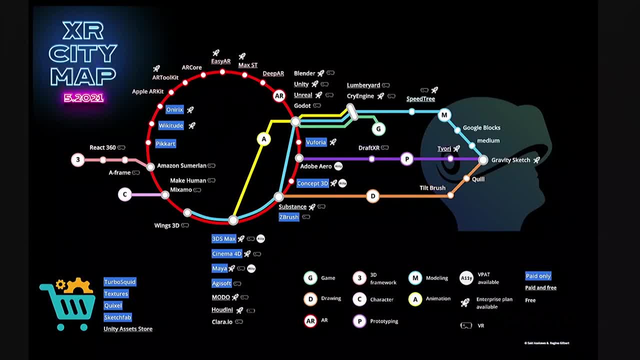 It guides people and helps them to determine if they are going to use what tool when. So I will just read the legend. There is a map here which appears to be a subway map. There's a lane for gaming, for drawing, for AR, for 3D frameworks for characters, for prototyping, for modeling. 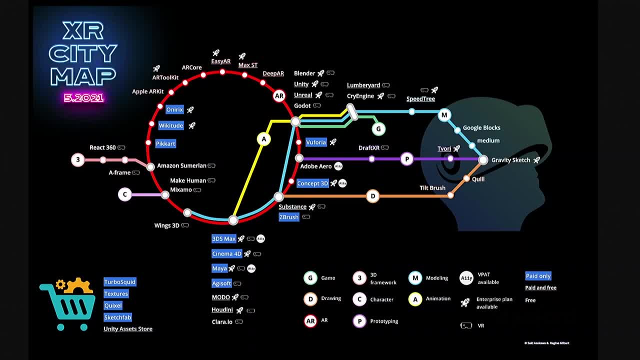 for animation, And one of the things that was important for us is: are things free? Are they free or not? Because that's again a barrier to entry. And then, is there any sort of accessibility documentation related to any of these tools Out of the 60 plus? we looked at how. 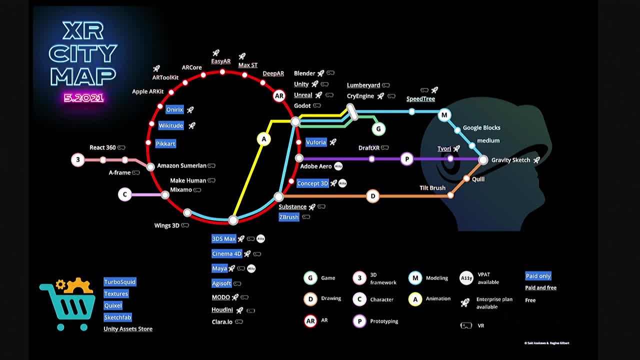 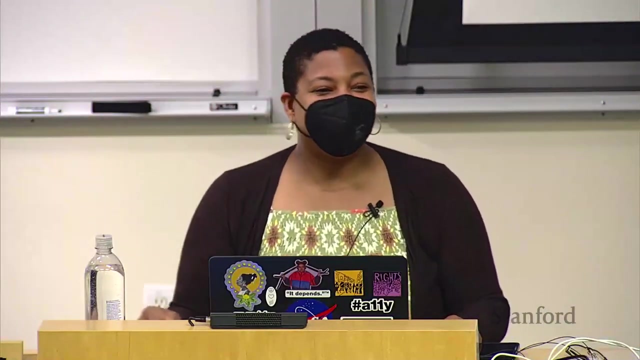 many do you think had any sort of accessibility documentation with them? Looked at 60, over 60, how many had accessibility documentation? I'm seeing number three. I see number four. I see a lot of threes, Three, Three. Somebody's saying zero, Two, Four, Four. So there's a gap there. 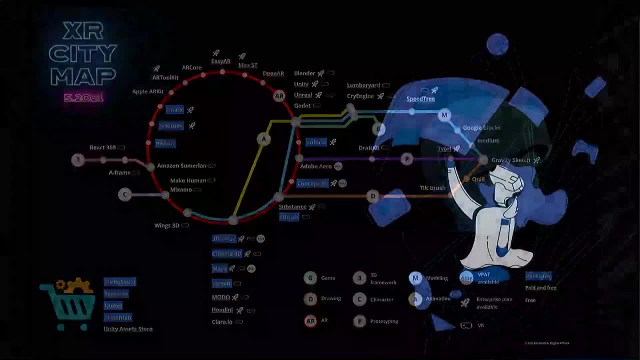 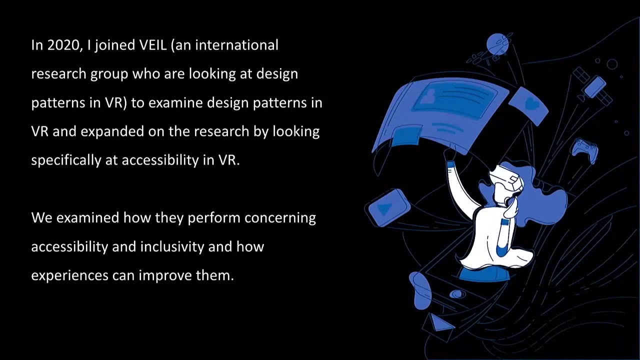 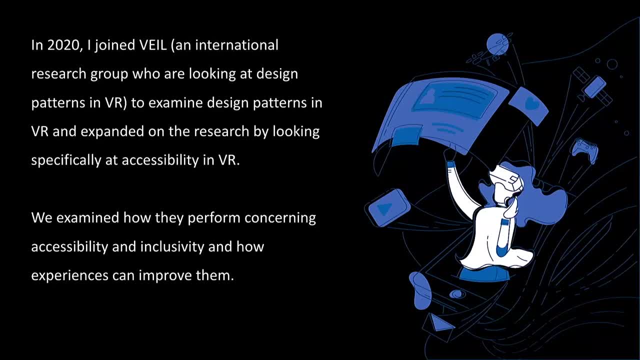 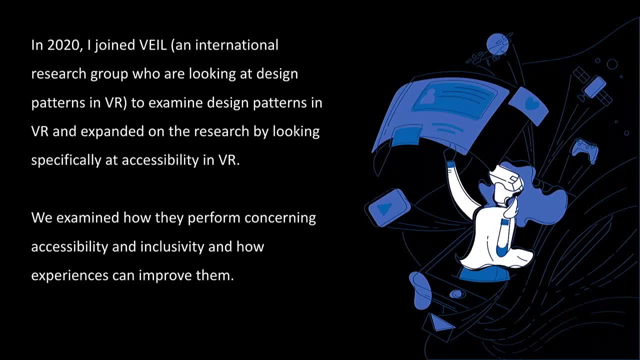 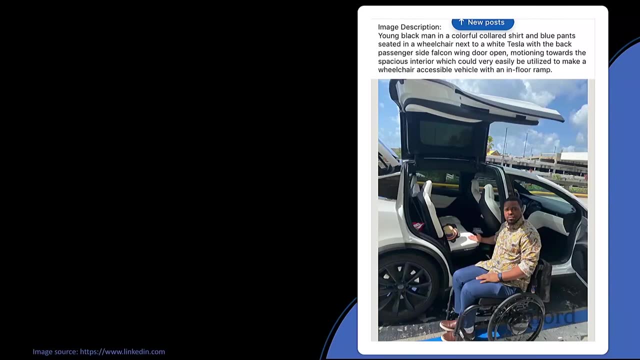 who is my grad research assistant last summer. So we examined how they perform concerning accessibility and inclusivity and how experiences can improve them. So here is an image description: A young black man in a colorful collared shirt and blue pants seated in a wheelchair next to a white Tesla with a black passenger side falcon wing door open, motioning towards a spacious interior which could very easily be utilized to make a wheelchair accessible vehicle with an in-floor ramp. How do you think this person could get into this vehicle? 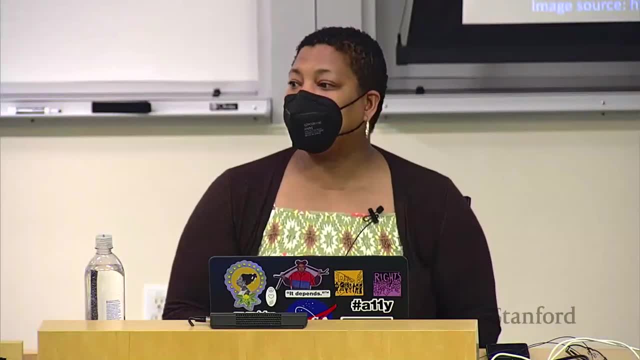 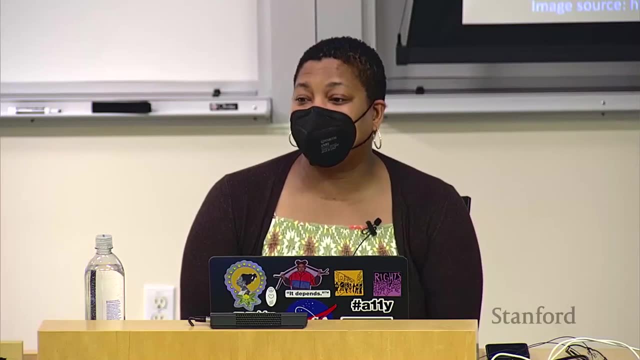 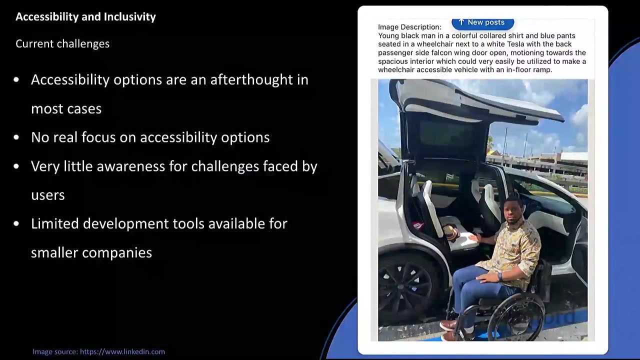 More importantly, why isn't there a ramp? It adds to the cost. It adds to the cost. Yes, They just didn't think about it. They didn't think about it. Yet again, they didn't think about it, right. So you know there are some current challenges. right, Accessibility options are an afterthought in most cases. right, And this is in reference to VR. 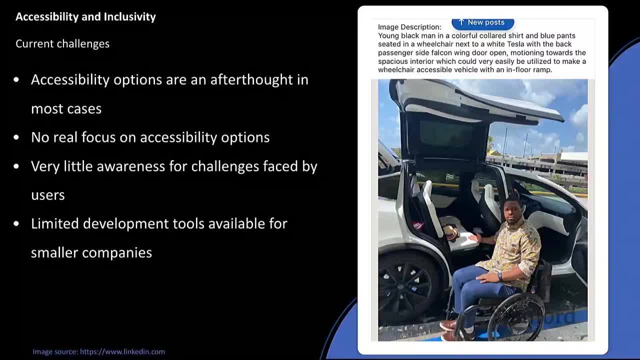 But it's also in reference to life. There's no real focus on accessibility options, There's very little awareness for challenges faced by users And there's limited development tools available for smaller companies. I want to tell this story real quick. I got asked. someone reached out to me to speak to me about accessibility in the XR space and they had made a video about accessibility in VR. 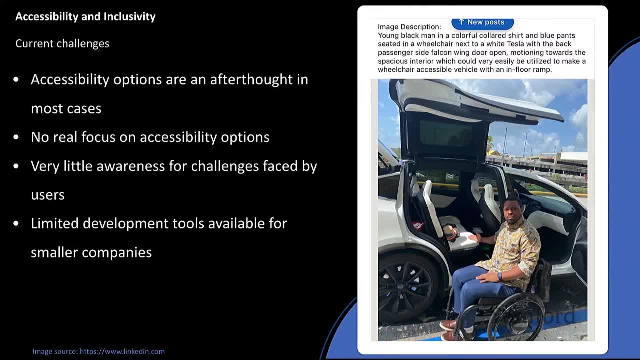 And they had made a video about accessibility in VR. And they had made a video about accessibility in VR And I went to watch the video and the video did not have any captions. Which, why? Why not right? That's a huge deal. If you make a video, add captions, YouTube like automatically has them. You can adjust them. 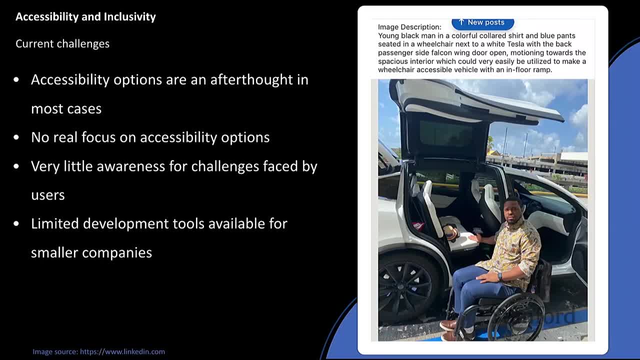 And when I asked this person why did you not add captions to the video that you made about accessibility, they told me because it would take too long. What can I say? What can I say, Except I did say a lot of things. 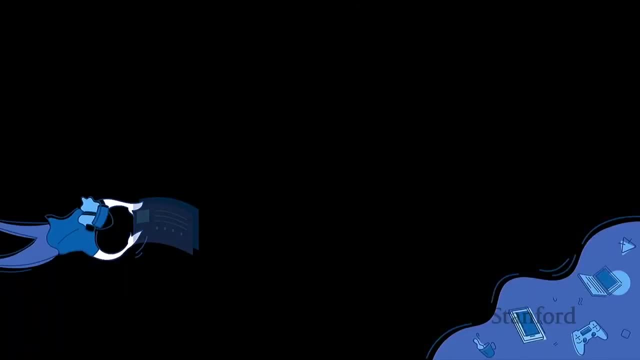 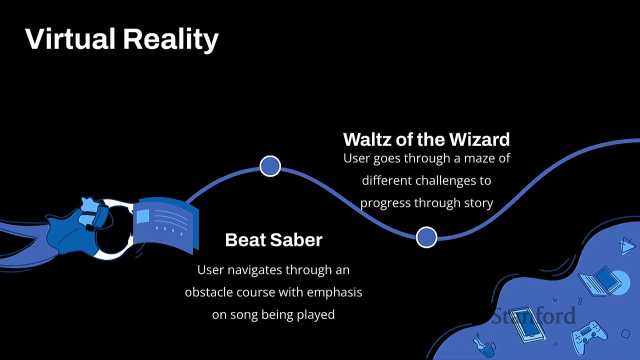 So with that, here I have a bit of an animation of the different titles that we tried for virtual reality. Any Beat Saber users in the house? Beat Saber user? yeah, boom, boom, boom. It's a lot of fun. 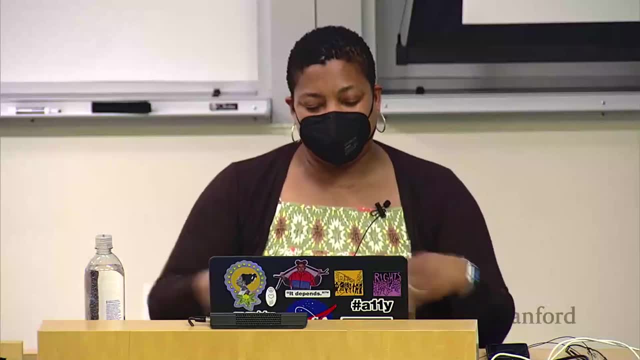 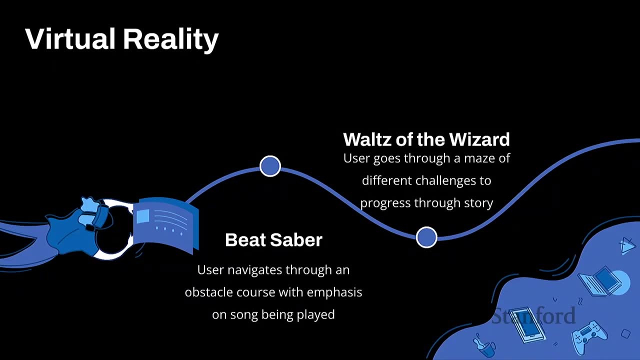 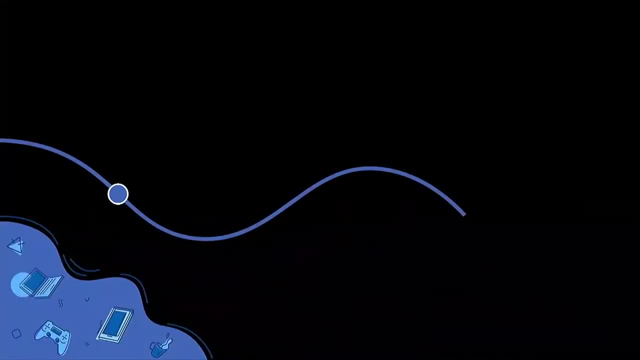 So Beat Saber, users navigate through an obstacle course With emphasis on the song being played right. Also, we tried Waltz of Wizard, where the user goes through a maze of different challenges to progress through a story. Here my animation continues with the different types of titles we used. 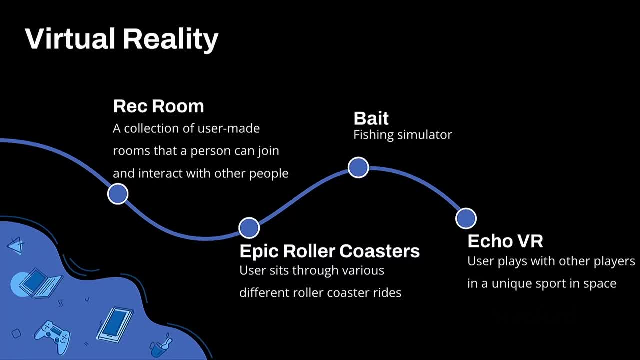 We used Rec Room, a collection of user-made rooms that a person can join and interact with other people. Epic Roller Coasters. If anybody has never tried VR before, don't do roller coasters. Roller coasters is your first experience. Don't do it. 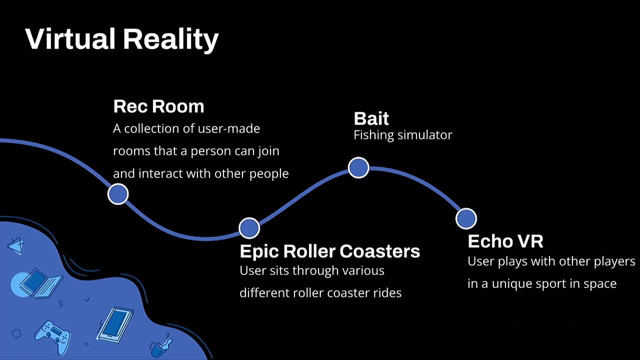 And if you do a roller coaster, please be seated. I'll just say that. So the user sits through various different roller coaster rides: Bait is a fishing simulator And Echo VR, where a user plays with other players in a unique sport and space. 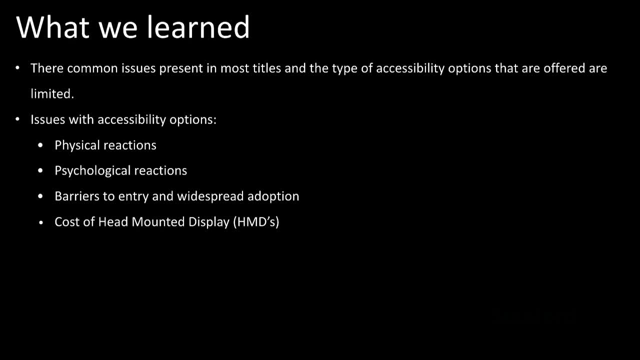 So what we learned were there were common issues present And in most titles, and the type of accessibility options that are offered are limited. Issues with accessibility options were physical reactions, psychological reactions, barriers to entry and widespread adoption and the cost of head-mounted displays. 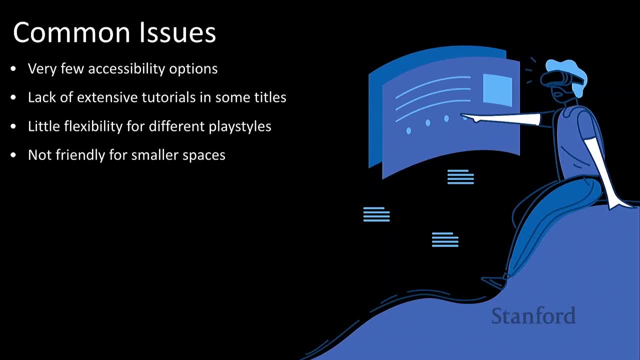 So here on the left I have an image of a person who's pointing with a VR headset on. So the common issues: very few accessibility options, a lack of extensive tutorials, Some titles, little flexibility for different play styles and not friendly for smaller spaces. 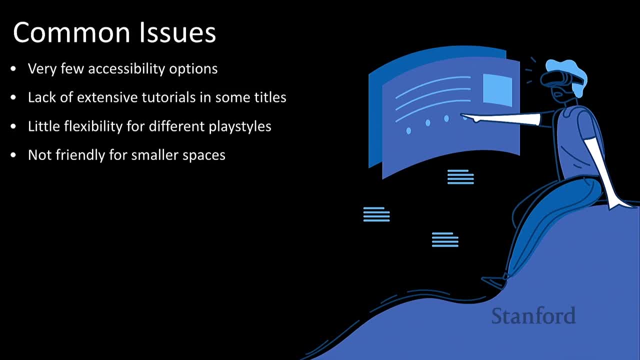 I live in Brooklyn. Literally, my couch and my refrigerator are like this, close right, Like so. I don't know who created these games or what spaces they use, but they were not in a Brooklyn apartment Because, although with the Quest 2, which is what we use, you can create a boundary, I had to be super careful. 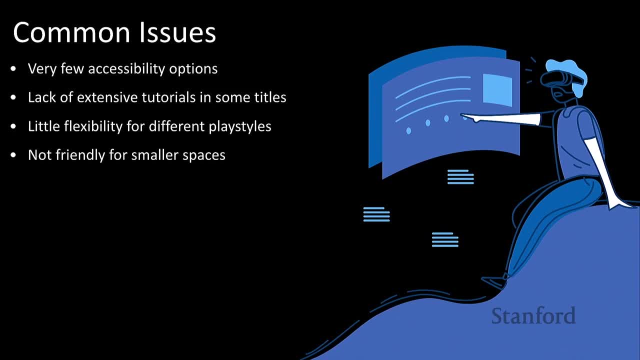 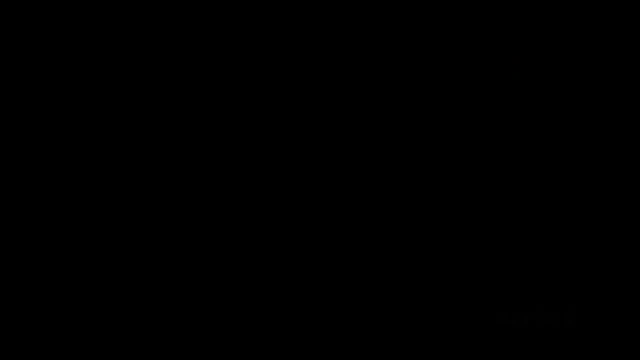 Not to hurt myself and, as a matter of fact, I don't like really doing VR in my apartment anymore at all. I prefer like my office, which has a lot more space. So some of the accessibility options are hand tracking. 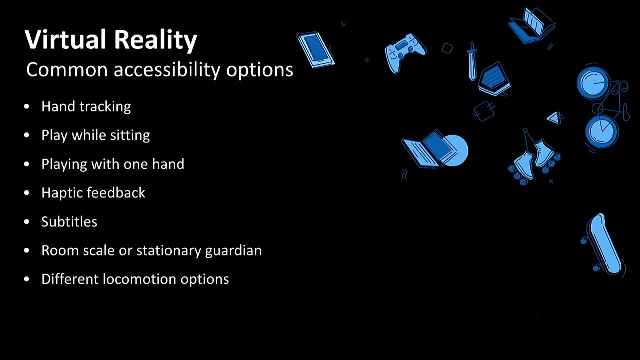 Has anyone tried the hand tracking with Quest 2? It's improving slowly. Playing while sitting playing with one hand: haptic feedback, subtitles, room scale, and so on. Playing while sitting playing with one hand: haptic feedback, subtitles, room scale, and so on. 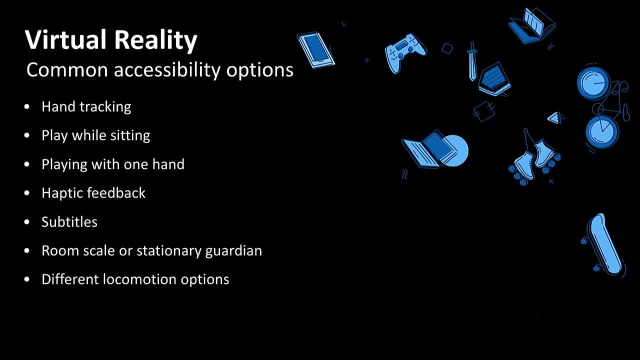 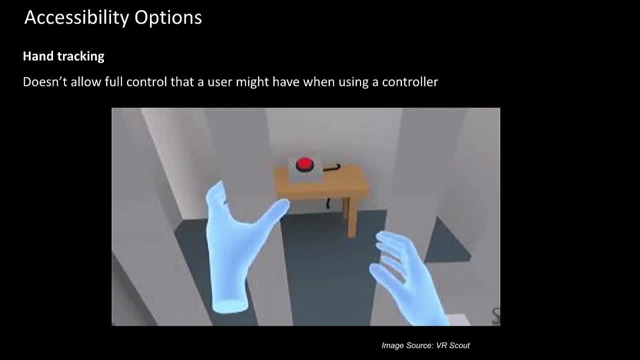 Or maybe held transaction. I also have a game called the Chrome Engine, I would say. starting at 1 am with work for a female player, I set the walkie-talkies at a stop of five blocks away monitor during the day, so I canオny place but not finish today. 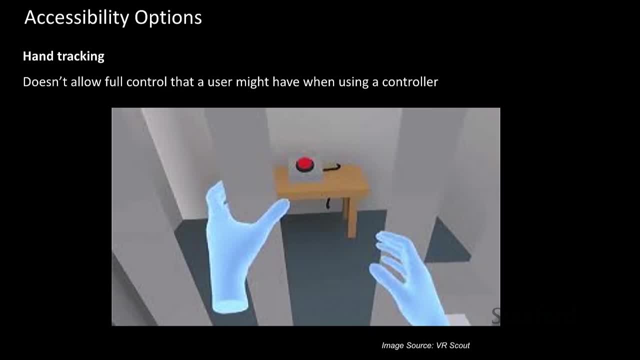 I also have a mobile gaming controller, which I consider fee-azucks because there'sparce for an edge. So, as I said in the talk earlier, I played and shadow lagged both for the Teams and other games, but also anything that works. 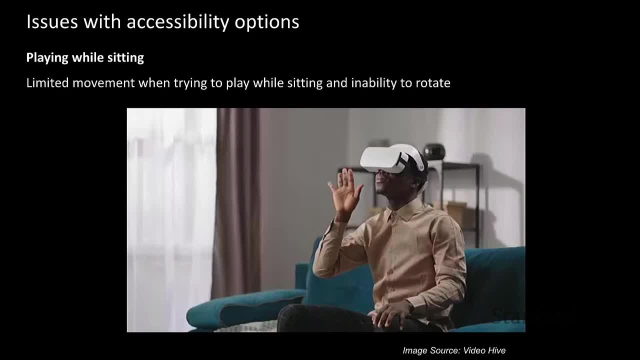 The other things that are working and I'm gonna look at on the computer, on the control tower right now is again video games, Because they work with Windows, trying to play while sitting and inability to rotate, So a lot of the experiences if you wanted to sit. 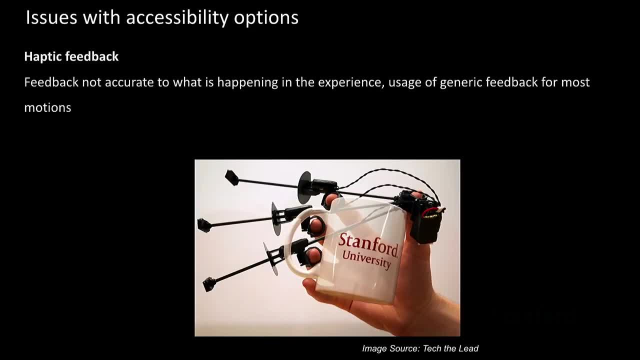 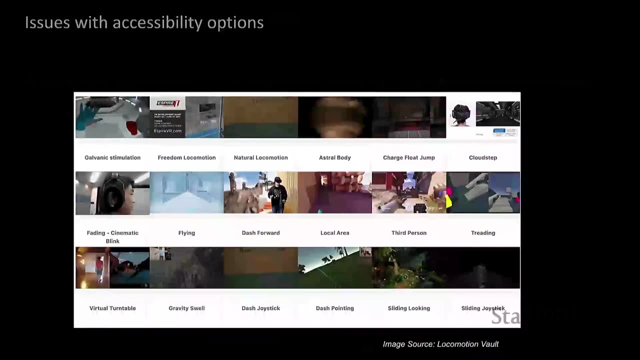 it wasn't the best for your gameplay. I had to throw this Stanford cup in here because I'm here, So for haptic feedback, feedback not accurate to what is happening in the experience and usage of generic feedback for most motions, And this is a great resource for those. 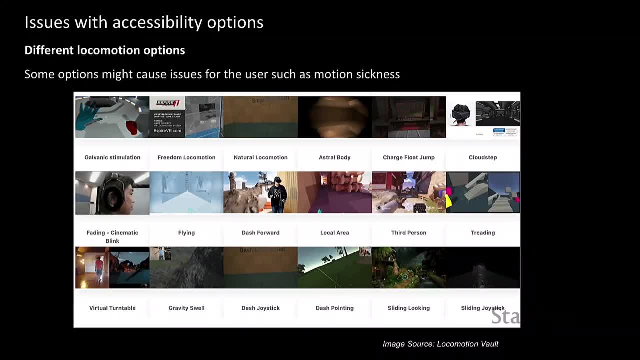 who are interested in learning more about VR. This is on GitHub. This is called the locomotion vault. I will say this: if you have motion sickness to things that move, this might do something to you, because they have all these gifts that are moving. 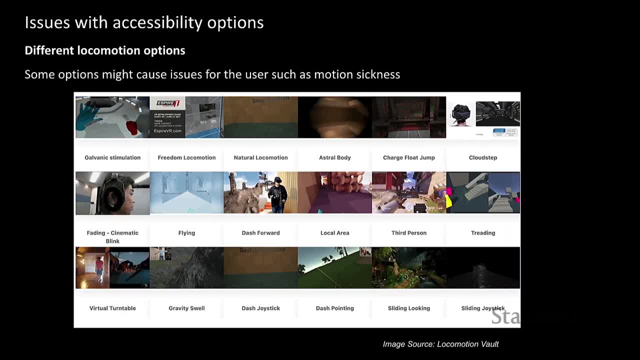 So I'll just say that as a warning when you go into the GitHub. But some options might cause issues for the user, such as motion sickness, which a lot of people still get with VR experiences, And this is something that Asad pointed out. 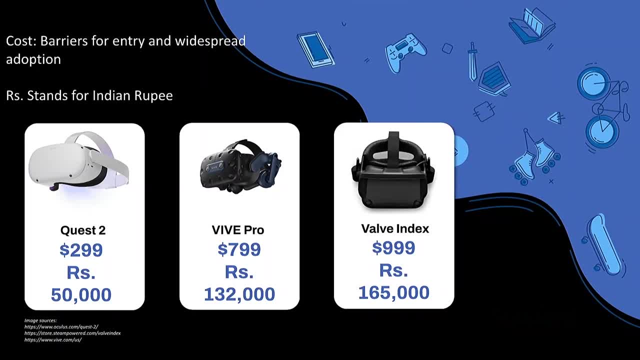 The cost is a barrier. So RS here stands for Indian rupee. On the left-hand side I have a Quest 2, which is $299, but it's 50,000 rupee. In the middle is a Vive Pro $799, 132,000 rupee. 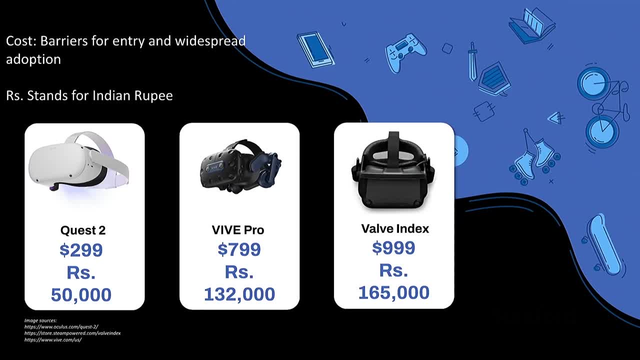 And on the right-hand side is a Valve Index: It's $999.. And a Vive Pro- $799.. 165,000 rupee. So I had a conversation with someone in India a few months back and they had just ordered a Quest 2. 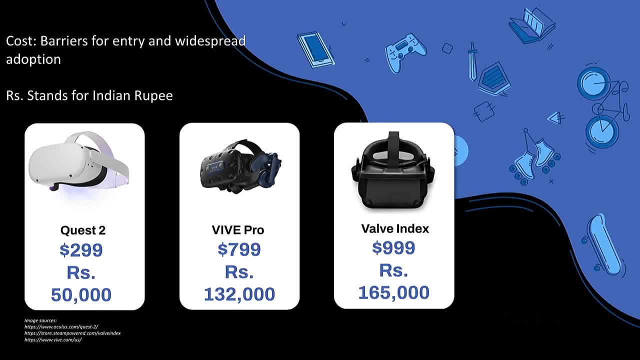 and said it was one month's salary. So for me that's like: well, if everybody's talking about it, I'm not going to say the M word, But if everybody's talking about the M word, you all know what the M word is. 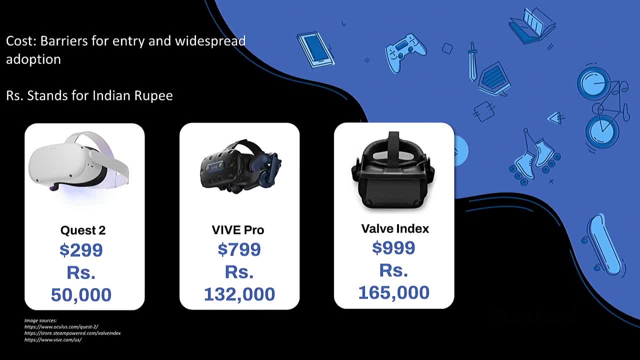 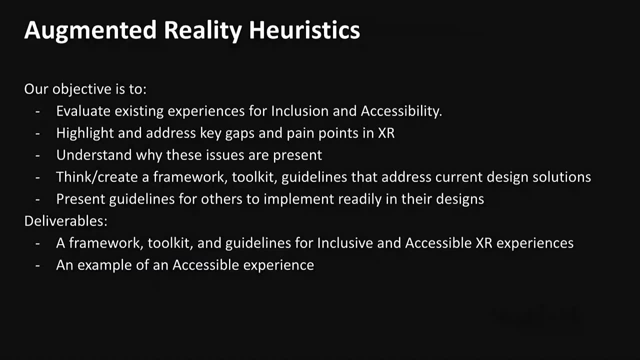 If everybody's talking about this being the next big thing, is it really? Because? who is this for Right? So another thing I'm working on currently is augmented reality heuristics. So our objective is to evaluate existing experiences for inclusion and accessibility, highlight and address. 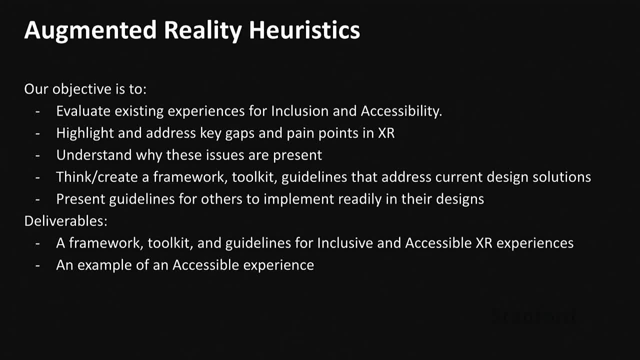 key gaps and pain points in XR in general, understand why these issues are present, and think and create a framework toolkit, guidelines that address current design solutions and present guidelines for others to implement readily in their designs And our deliverables- we hope by the end of this year. 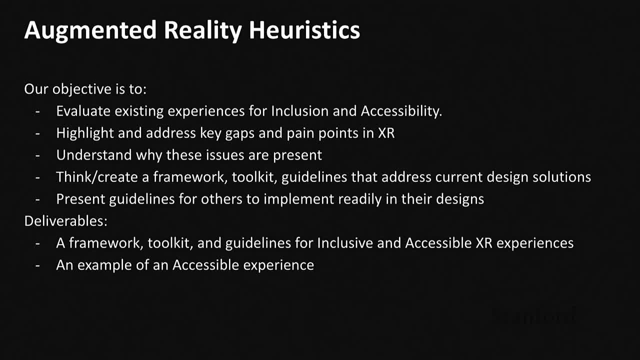 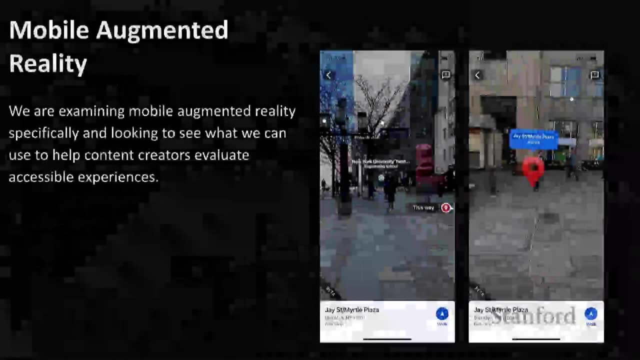 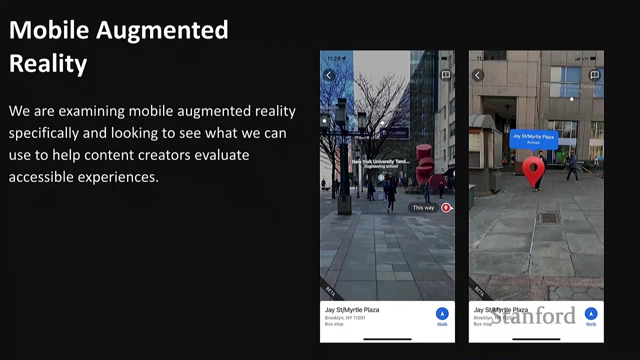 to have a framework toolkit and guidelines for inclusive and accessible XR experiences from a content creator perspective, from a designer and developer perspective, and an actual example of an accessible experience. So this here on the right, I have two images of using Google Maps. 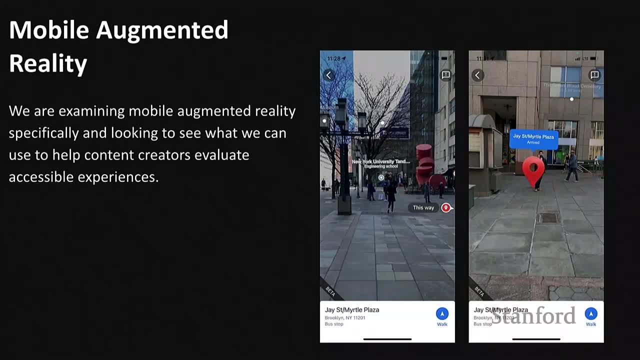 and this is a beta version of augmented reality. This is near my campus and I got a group of students to use this and get some good feedback on what they saw. So we're examining mobile augmented reality specifically and looking to see what we can use to help content creators evaluate. 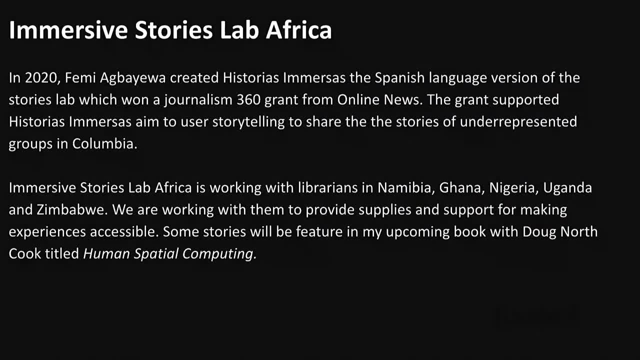 accessible experiences, And this is another part of my ongoing research- is working with Immersive Stories, Lab Africa In 2020,, and I want to make sure I say Femi's name correctly: Femi Agbaweya created Historias Inmersas. 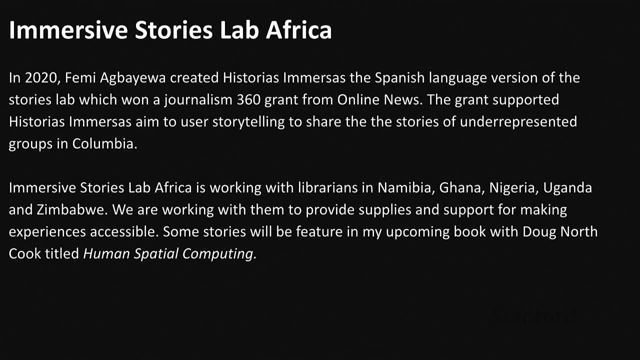 the Spanish language version of the Stories Lab, which won a journalism 360 degree 360 grant from online news. The grant supported Historias Inmersas' aim to user storytelling, to share the stories of underrepresented groups in Colombia. So Immersive, Story Lab Africa is working with libraries. 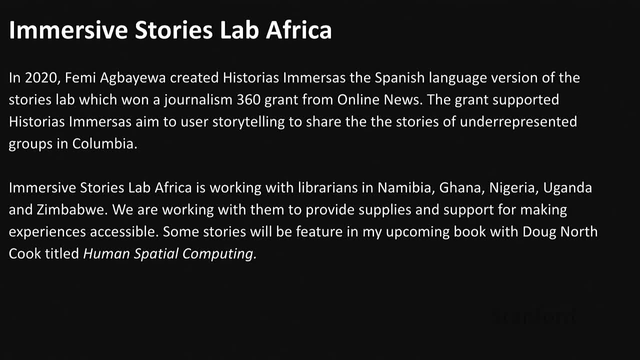 librarians in Namibia, Ghana, Nigeria, Uganda and Zimbabwe. We- my team- are working with them to provide supplies and support for making experiences accessible. Some stories will be featured in my upcoming book, which I'm writing with Doug Northcook, titled Human Spatial Computing. 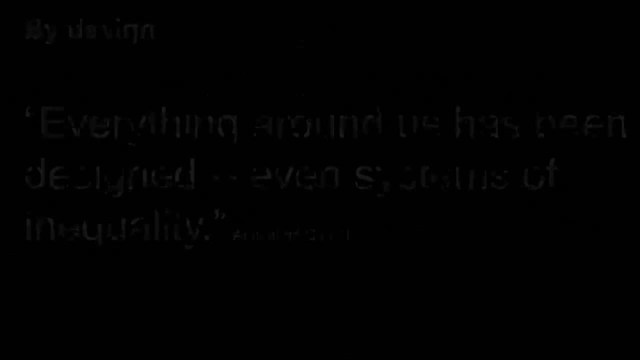 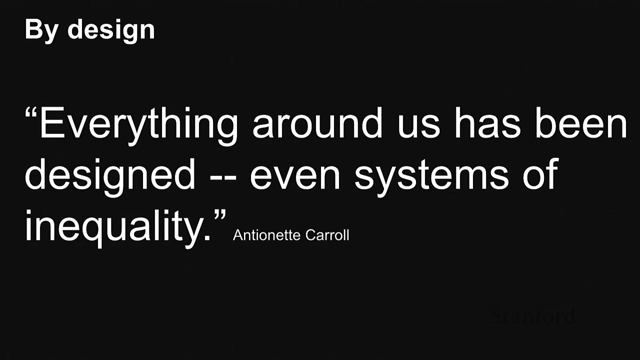 which will be coming out next year. So this is something for everybody to think about. Everything around us has been designed, even systems of inequality. We have an opportunity when working on these technologies, to make things a little bit better, And this is a quote from Antoinette Carroll. 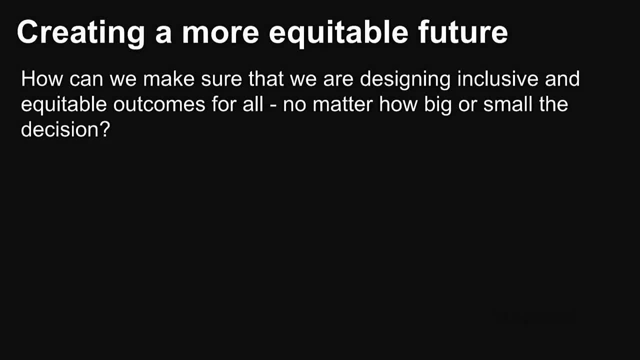 who is an amazing human, So thinking about creating a more equitable future. how can we make sure that we are designing inclusive and equitable outcomes for all, no matter how big or small the decision? This is for each of you to think about individually. 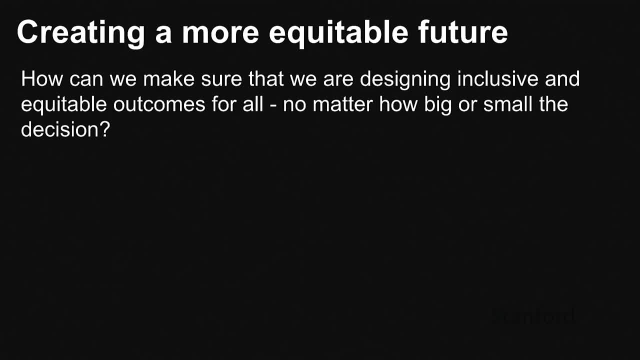 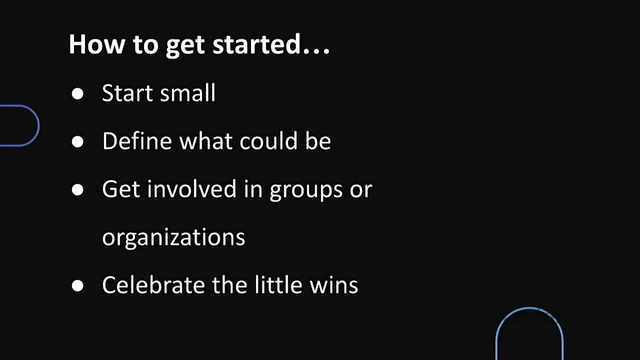 How can we make sure that we are designing inclusive and equitable outcomes for all, no matter how big or small the decision, whether you're working on a class project or you're working somewhere, So how you can get started. start small, define what could be. 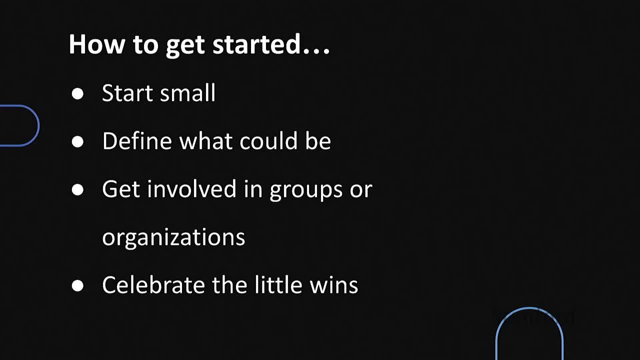 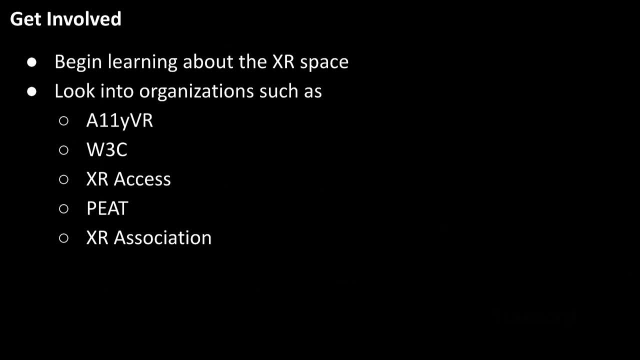 get involved in groups or organizations and celebrate the little wins. So begin learning about the XR space if you have interest. I think everybody should, because it's pretty cool to get interested in this And look into organizations such as A11Y-VR, the W3C, XR Access. 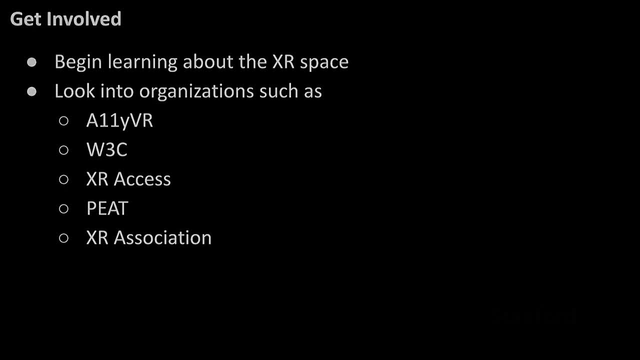 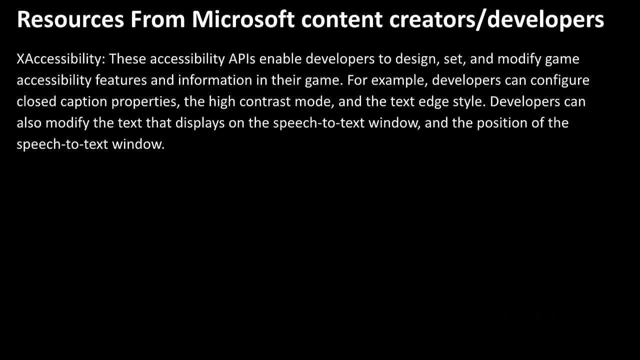 PEAT XR Association. All right, Thank you, So I'm going to cover a few of them. Oh, first. so this is for you back there, because you're my developer. Everyone else, if you want to take a nap, you might. 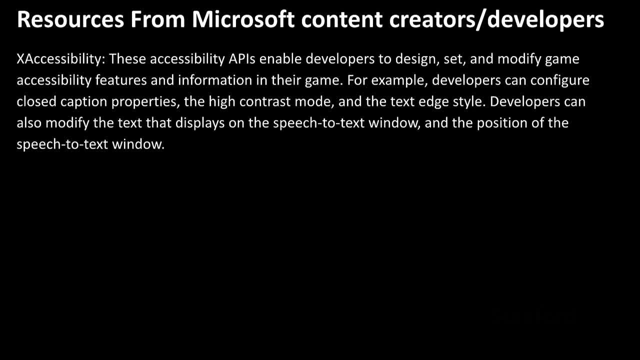 But it's OK. So these are some resources from Microsoft for content creators and developers. So X accessibility. These accessibility APIs enable developers to design, set and modify game accessibility features and information in their game or VR experience. For example, developers can configure closed caption. 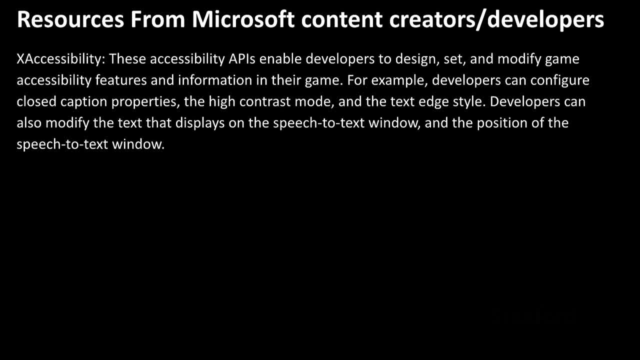 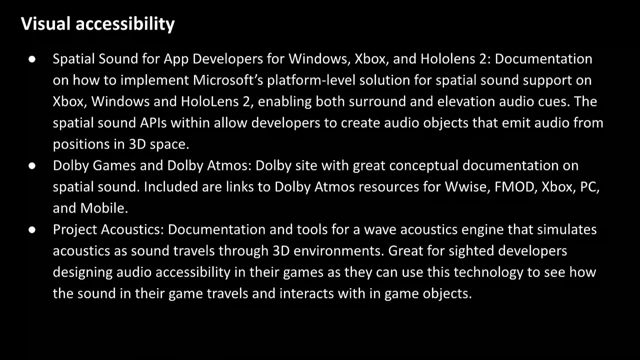 properties, the high contrast mode and the text edge style. Developers can also modify the text that displays on the speech-to-text window and the position of the speech-to-text window. For visual accessibility, there's spatial sound for app developers for Windows, Xbox and HoloLens 2.0.. 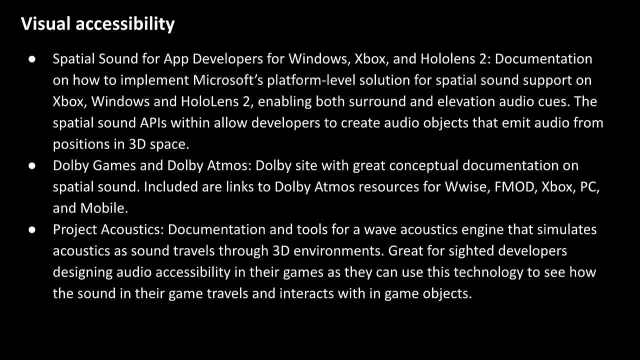 Documentation: Documentation on how to implement Microsoft's platform level solution for spatial sound support on Xbox, Windows and HoloLens 2.0, enabling both surround and elevation audio cues. The spatial sound APIs within allow developers to create audio objects that emit audio. 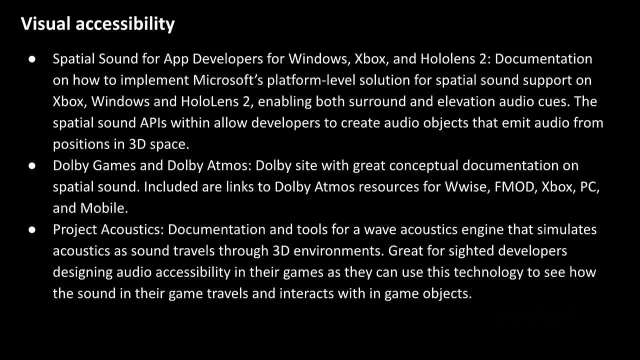 from positions in 3D space. Dolby Games and Dolby Atmos- Dolby's site with great conceptual documentation on spatial sound, included our links to Dolby Atmos. resources for W-W-I-S-E- I'm just spelling it out: F-M-O-D, Xbox, PC and mobile. 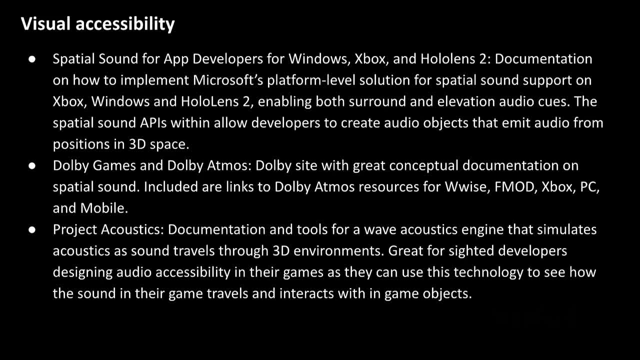 Project acoustics documentation and tools for Wave Acoustics Engine that simulates acoustics as sound travels through 3D environments. It's great for sighted developers designing audio accessibility in their games, as they can use this technology To see how the sound in their game travels and interacts. 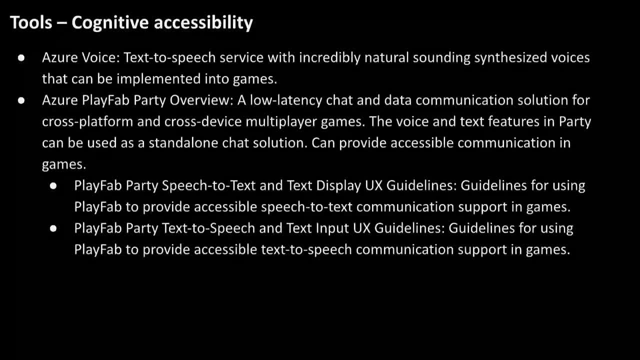 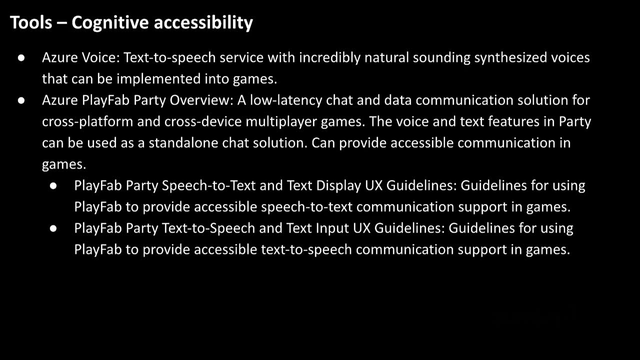 with within game objects. I love that you're paying attention. I'm just focusing on you back there. All right tools, Cognitive accessibility. So Azure Voice text-to-speech service with incredibly natural sounding synthesized voices that can be implemented into games. 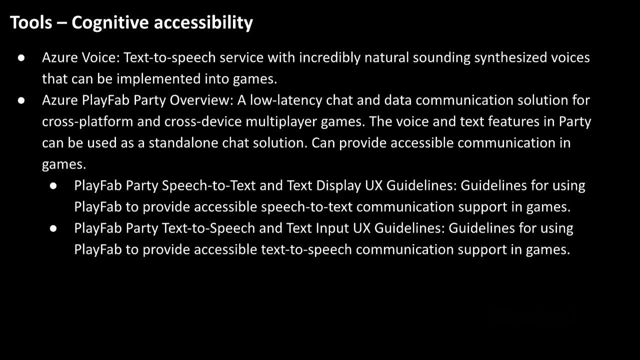 Azure PlayFab Party Overview: a low latency chat and data communication solution for cross-platform and cross-device multiplayer games. The voice and text features in Party can be used as a standalone chat solution and can provide accessible communication in games. So PlayFab Party Speech-to-Text and Text Display UX Guidelines. 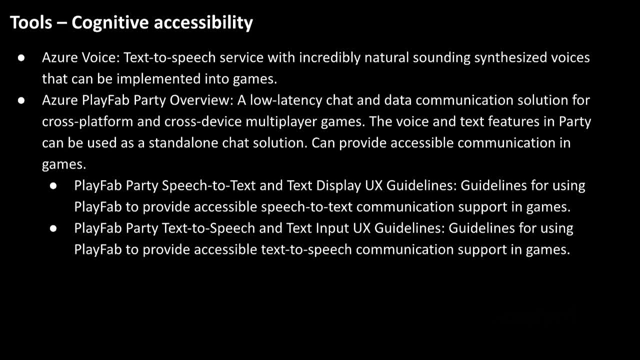 for using Guidelines for Using PlayFab to provide accessible speech-to-text communication support in games. There's also PlayFab Party Text-to-Speech- say that five times fast and Text Input UX Guidelines. So Guidelines for using PlayFab to provide 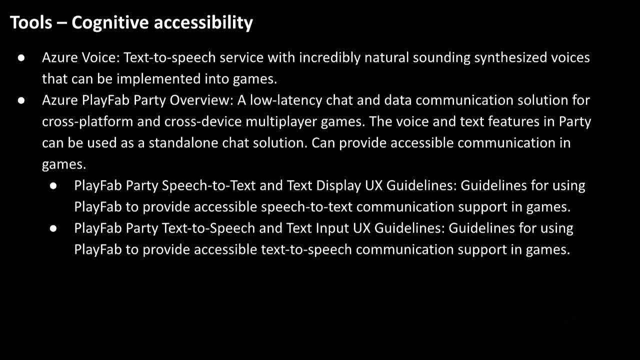 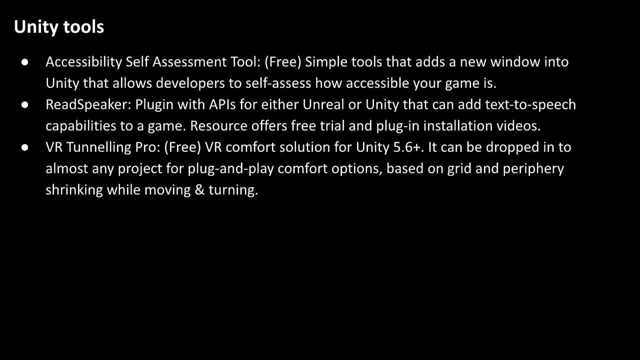 accessible text-to-speech communication. support in games For Unity. where my Unity Unity. So there's Accessibility Self-Assessment Tool, which is free, Simple tools that add a new window And to Unity that allows developers to self-assess how accessible your game is. 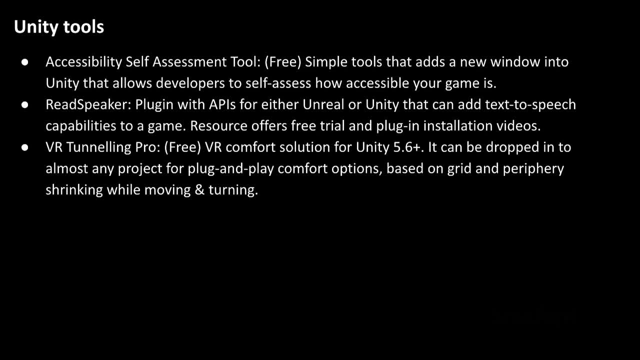 or your experience is ReadSpeaker, which is a plug-in with APIs for either Unreal or Unity that can add text-to-speech capabilities to a game. Resources offer free trial and plug-in installation videos. VR Tunneling Pro, which is also free. 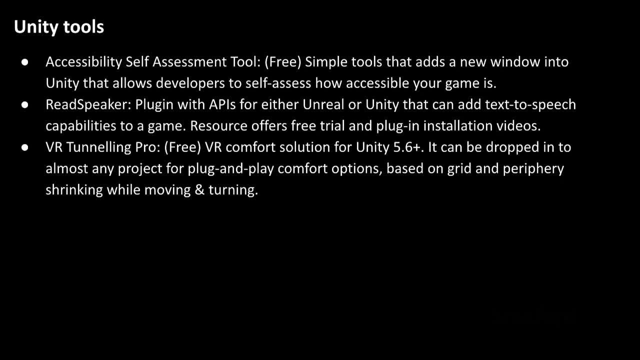 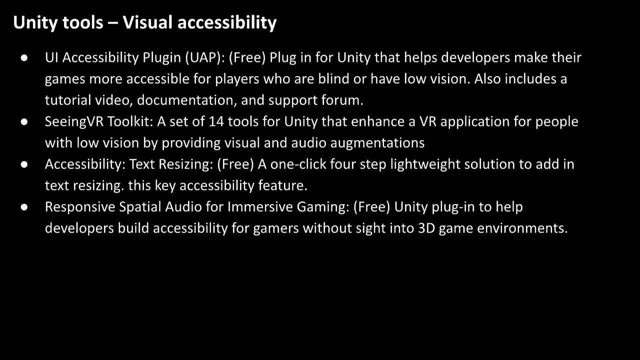 It's a VR comfort solution for Unity 5.6 and higher And it can be dropped into almost any project for plug-and-play comfort options based on grid and periphery shrinking while moving and turning. And here's some Unity tools for visual accessibility: 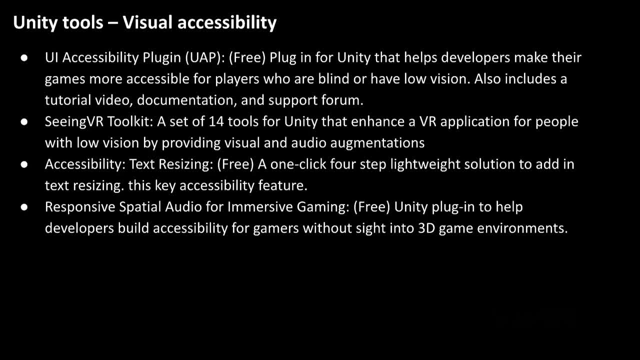 So there's UI Accessibility Plugin, UAP, which is also free Plug-in for Unity that helps developers make their games more accessible for players who are blind or have low vision. It also has a UI Accessibility Plugin, UAP, which is also free. 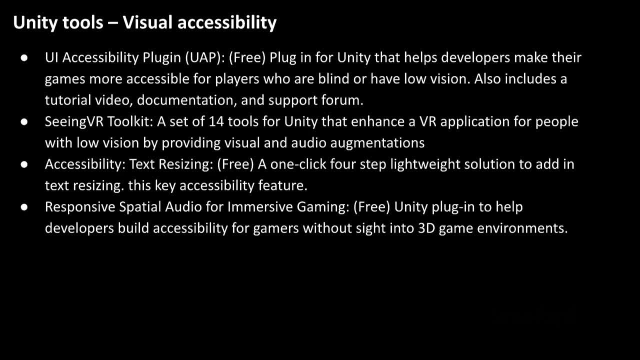 It also includes a tutorial video, documentation and support form. Seeing VR Toolkit. it's a set of 14 tools for Unity that enhance a VR application for people with low vision by providing visual and audio augmentations. There's Accessibility- Text Resizing, which is free. 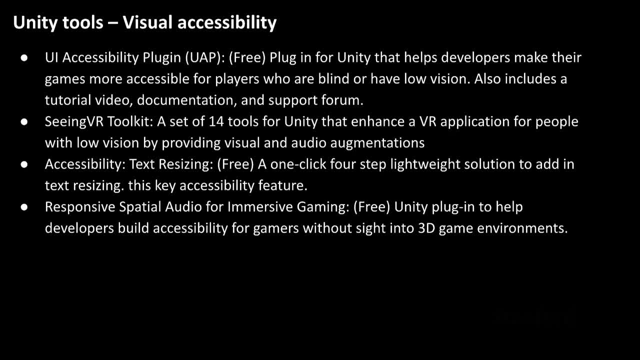 It's a one-click, four-step lightweight solution to add in text resizing- This is a key accessibility feature- And Responsive Spatial Audio. So this is for immersive gaming: Free Unity Plugin to help developers build accessibility for gamers without sight into 3D game environments. 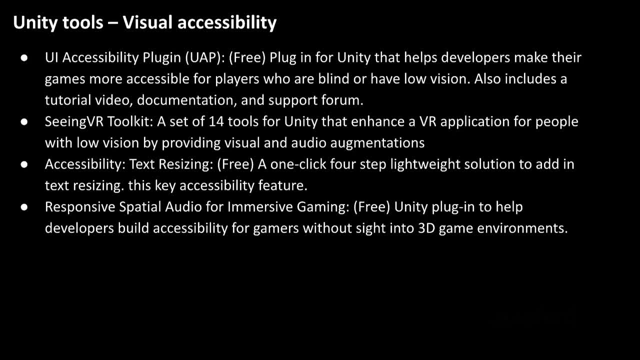 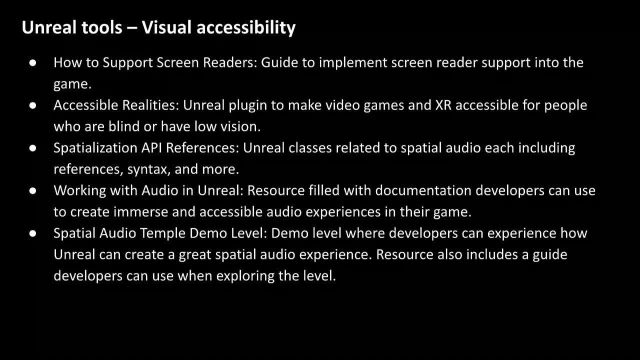 Did any of you know about these? my Unity people? No OK, OK, cool, All right for Unreal, any Unreal people in the house? No OK. So for visual accessibility, how to support screen readers: guide to implement screen reader support into the game. 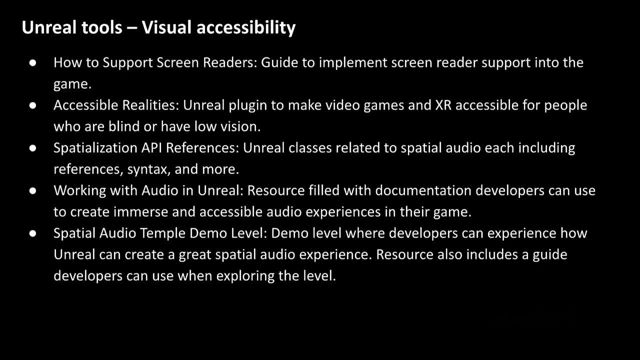 There is Accessible Realities Unreal Plugin to make video games and XR accessible for people who are blind or have low vision. Spatialization API references, so Unreal classes related to spatial audio, each including references, syntax and more Working with audio in Unreal. so it's. 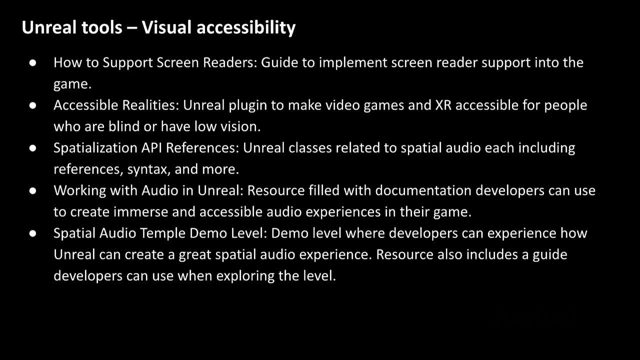 a resource filled with documentation developers can use to create immersed and accessible audio experiences in their game. Spatial audio temple demo level- so demo level where developers can experience how Unreal can create a great spatial audio experience. Resource also includes a guide developers can use when exploring the level. 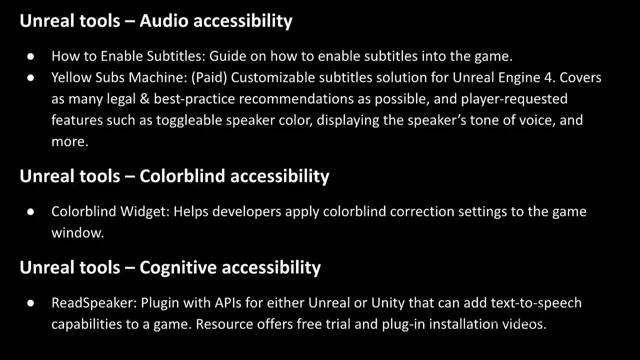 I'm almost through this, but I want to put it out there in the world. Unreal tools, so audio and accessibility. How to enable subtitles, so guide on how to enable subtitles into the game Yellow subs machine, which is a paid thing. it's not free. 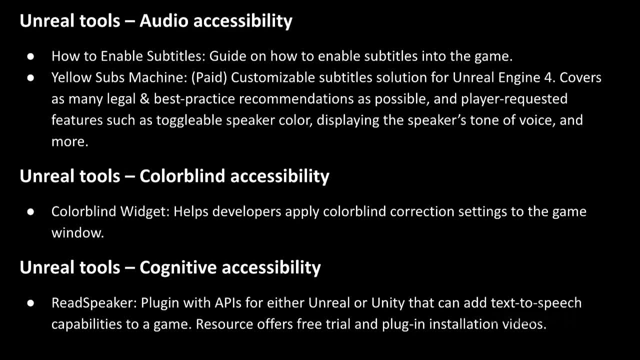 Customizable subtitle solution for Unreal Engine. 4. Covers as many legal and best practice recommendations as possible And player requested features, such as toggle- toggleable speaker color Displaying the speaker's tone of voice and more, And Unreal tools colorblind accessibility. 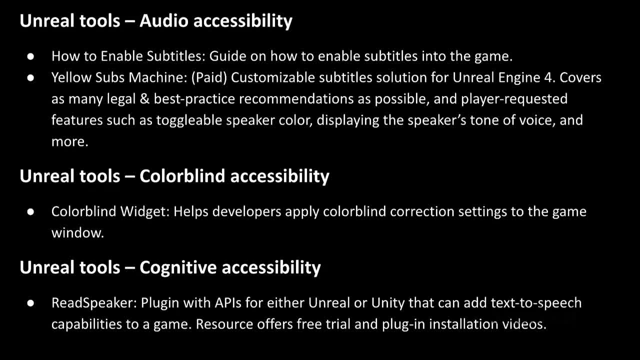 so there's a colorblind widget which helps developers apply colorblind correction settings to the game window And cognitive accessibility. so Read Speaker. a plug-in with APIs for either Unreal or Unity- I already mentioned this one That can add speech to text capabilities to a game. 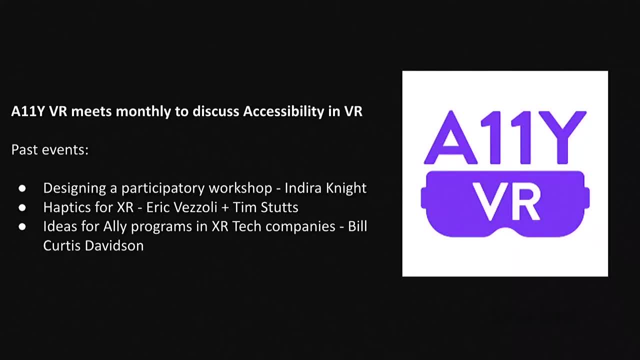 I made it through that, But I wanted to put that That out there in the world. So, for those of you who have interests in accessibility and VR, I recommend checking out the A11Y VR meetup. They meet monthly, but you can also. 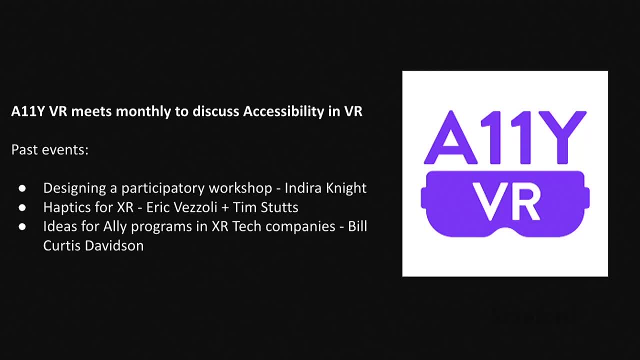 find previous past events on YouTube. Past events include designing a participatory workshop with Indira Knight. haptics for XR with Eric Vizzoli and Tim Stutz, And ideas- Ideas for ally programs in XR tech companies with Bill Curtis-Davidson. 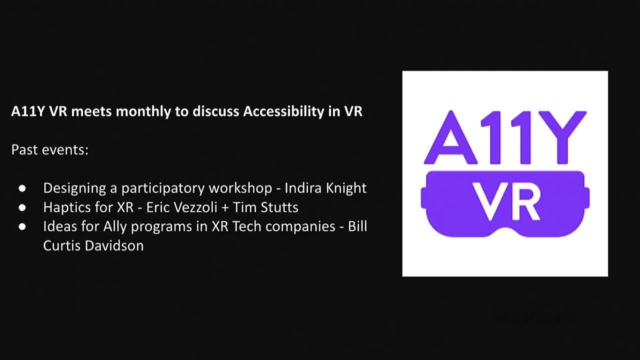 I have to ask this: Does anybody know what this stands for? A11Y, I know you do. You do OK. Anybody Who does not know what A11Y stands for? OK, A majority of this room, which means probably a majority. 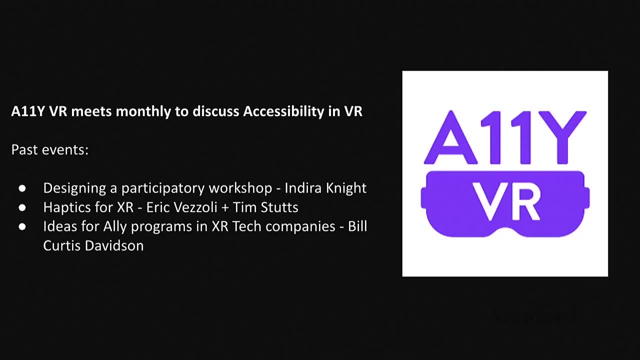 of people watching this. So A11Y is a numeronym for accessibility. There are 11 characters between the A And the Y, So if you have interest in learning more about accessibility, you can look up hashtag A11Y And you could find all kinds of stuff. 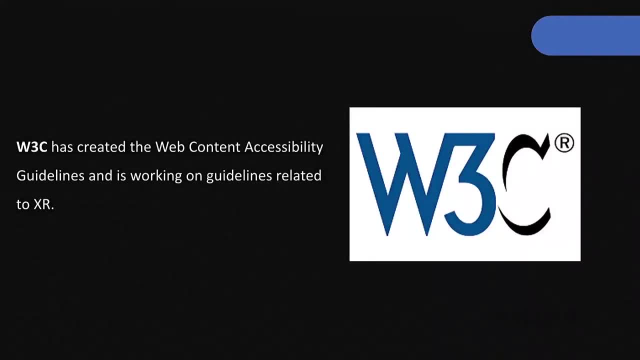 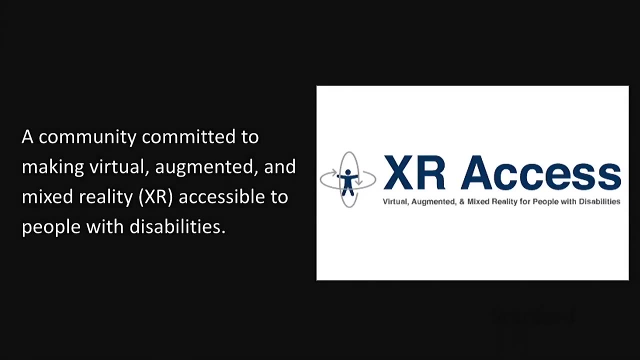 The W3C. you all know. now You Google it and you'll learn about it right, The W3C has created the web content accessibility guidelines And they're working on guidelines related to XR. There is XR access, Which I am a member of, a proud member of. 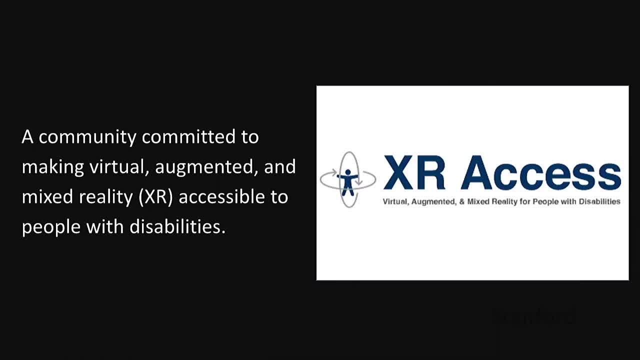 It's a community committed to making virtual, augmented and mixed reality accessible to people with disabilities. There is a symposium coming up. It'll be virtual this year in June, So if you're interested, go to xraxcessorg. It's a really wonderful, wonderful organization. 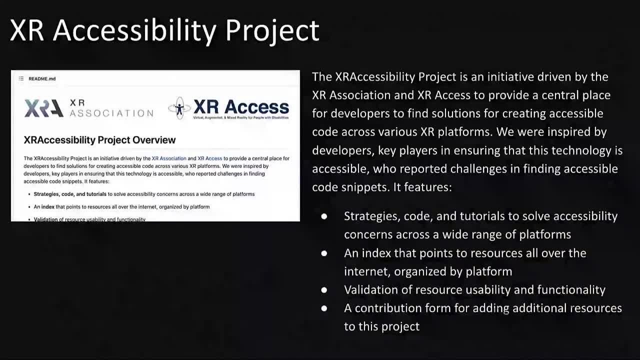 started by folks at Cornell Tech, So they also have this XR Accessibility Project. So the XR Accessibility Project is, I think, a little bit more than just a little bit. The XR Accessibility Project is an initiative driven by the XR Association and XR Access. 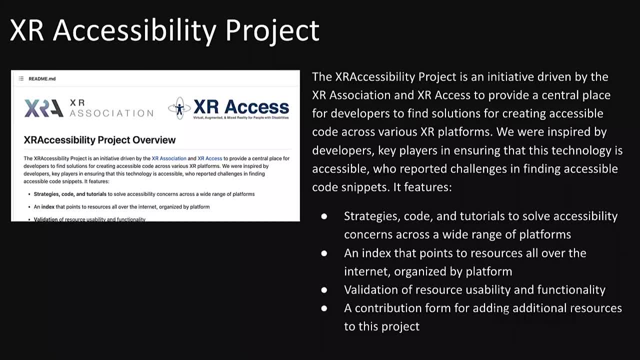 to provide a central place for developers and designers. I'll say that to find solutions for creating accessible code and strategy across various XR platforms. We were inspired by developers- key players in ensuring that this technology is accessible- Who reported challenges in finding accessible code. 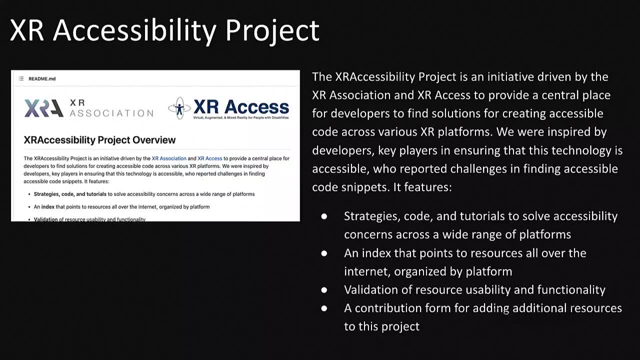 snippets, So it features a number of things. There's strategies, code and tutorials to solve accessibility problems across a wide range of platforms. an index that points to resources all over the internet organized by a platform. validation of resource usability and functionality. 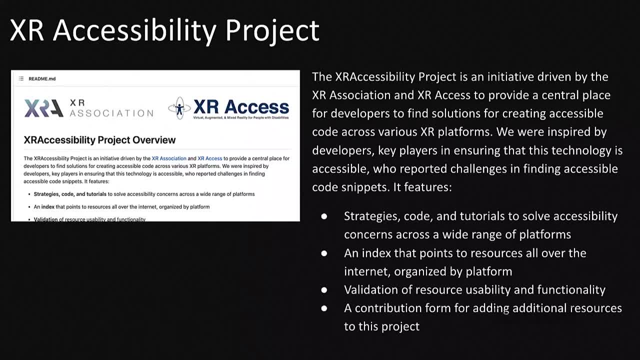 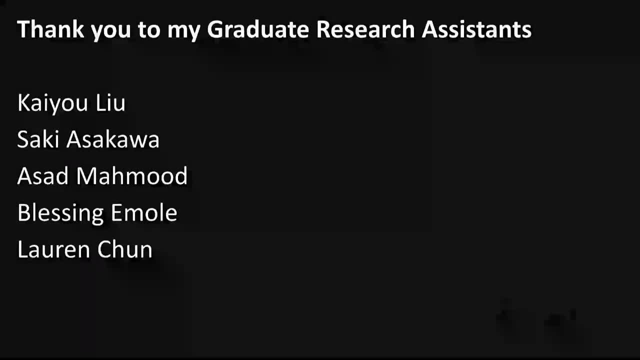 a contribution form for adding additional resources. So if you're interested and you're working on stuff, you can add to it to put it out there. open source. I want to publicly thank my grad assistant who I've worked with for the last few years. 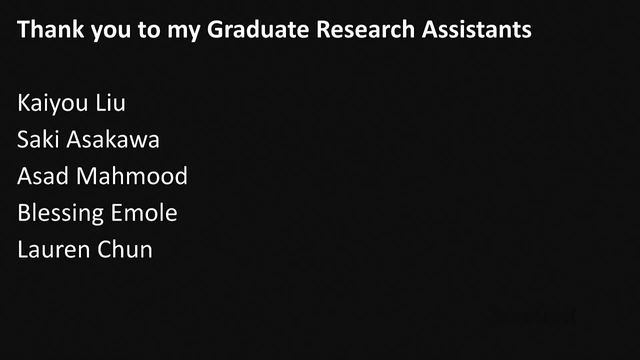 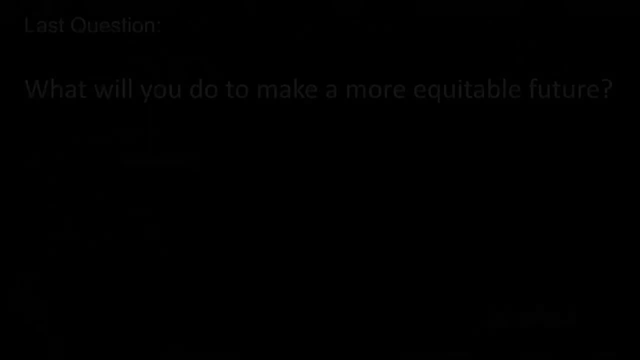 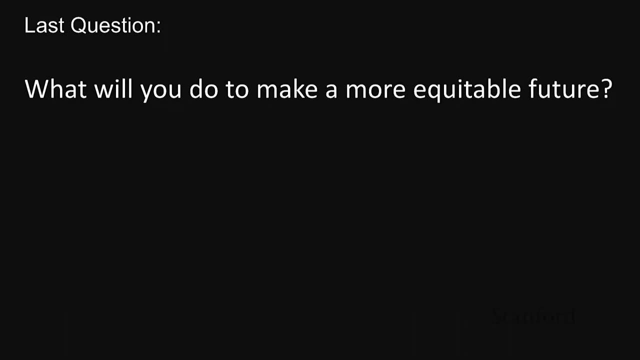 Kaiyu, Liu Saki Asakawa, Asad Mahmood, Blessing Amole and Lauren Chun. So thank you all. I appreciate you all so much, And my last question for all of you is: what will you do to make a more equitable future? 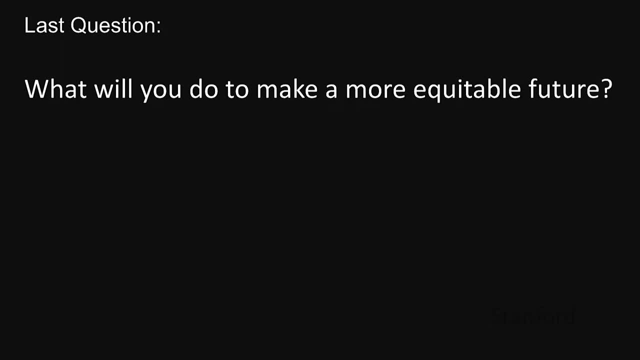 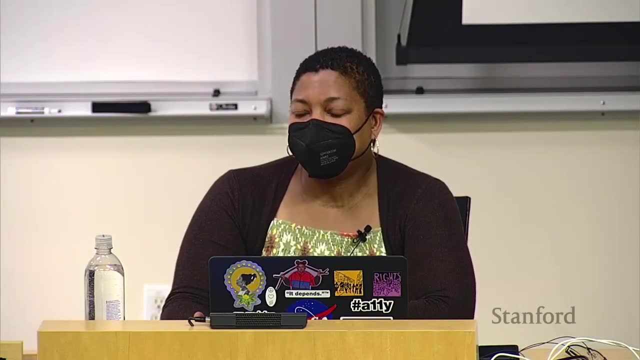 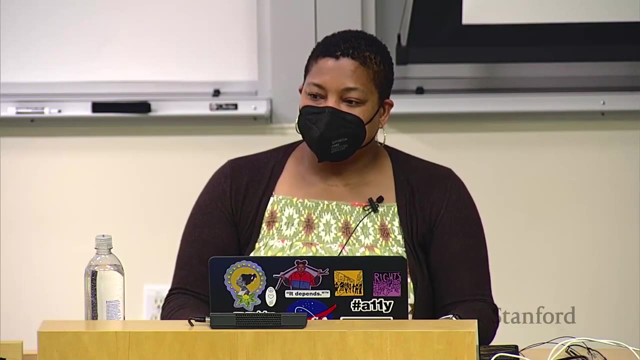 Anybody care to answer. So we've been really appreciating more students finding out about accessibility before they graduate, like offering more classes on accessibility so that they're prepared to think about that as they go out into the world to the working world. 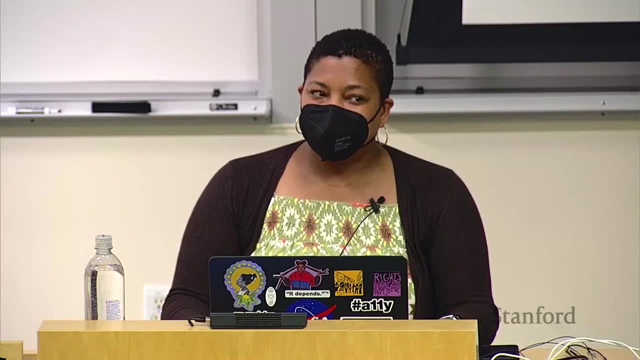 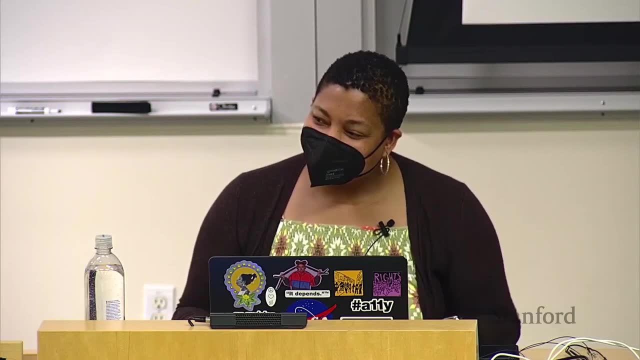 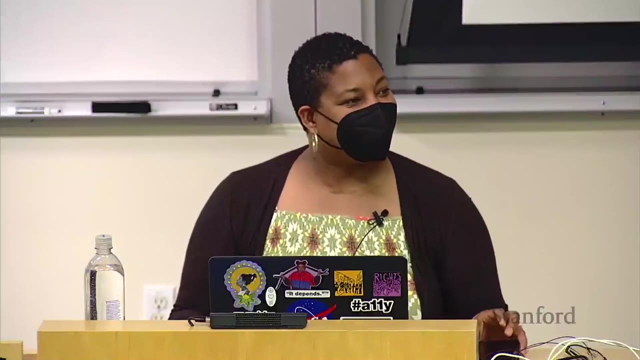 Yeah, Anyone else Suggest is: start small, Start small, Start small. Yes, Yes, Learning the tools and having a framework to understand how to start developing and designing with accessibility in mind before. So I'll just repeat what you said: learning the tools.